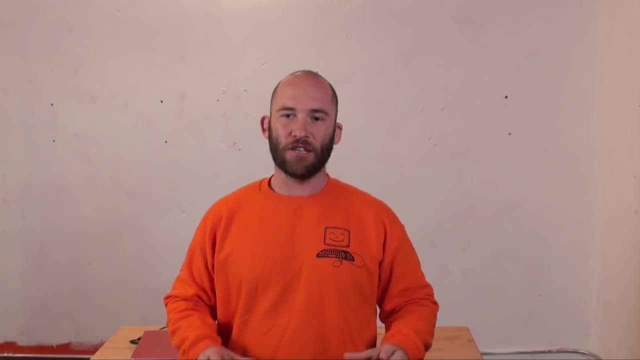 because they had to. But they didn't teach us about servers in general. They taught us very specifically about Windows servers, and Windows servers only. Well, as we are going into the server track, I want to give you a broader foundation on understanding how. 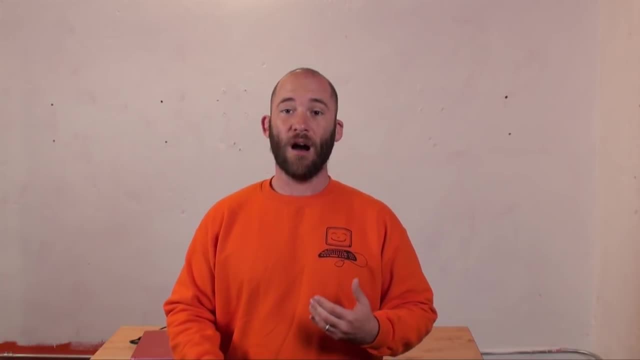 servers work. So in this class today, we are going to talk about a couple specific products, but we're going to talk more about the general idea of servers, what servers do in the network, what they provide to the clients on the network and things that you need to think about if 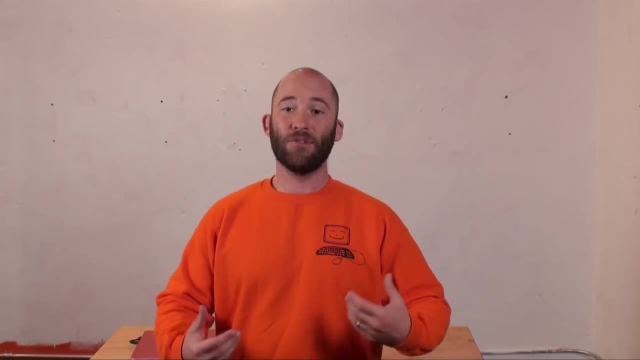 you're thinking about installing or if you have to maintain a server. So today's class on Introduction to Servers- Again, this is not specific- We're going to talk a little bit about Windows servers, a little bit about Linux servers. We're going to mention that. 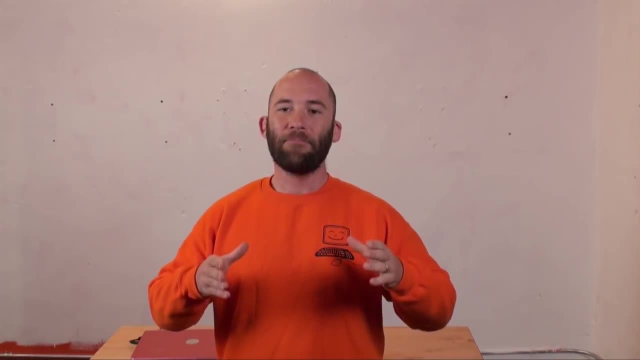 there's Mac servers out there. We're going to focus on those. This class is going to just be the overall idea of what is a server, why is it useful and what do you do with it. if you have one, So give me. 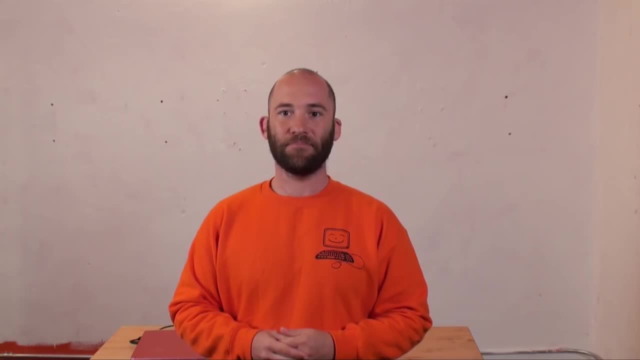 a couple minutes, I'll be back and we'll get into this class Now. the first thing that we have to do when we're talking about servers is we have to define what a server is. So a server is not simply: you know. if it has a server in the name, you know Windows. 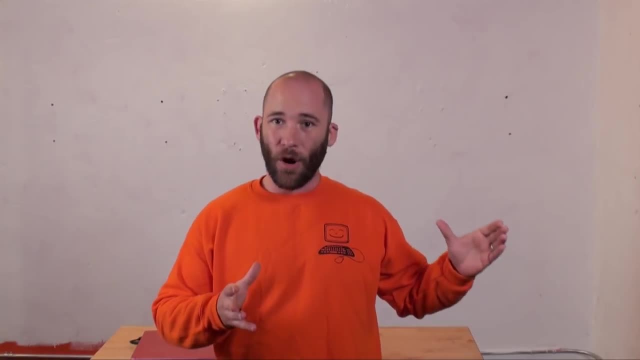 2008 server. That is a server, but that's not the only thing that can be a server. Basically, all a server is all a server is. this is nothing to be nervous about. all a server is it's a computer on a network that provides services to other computers on the network. 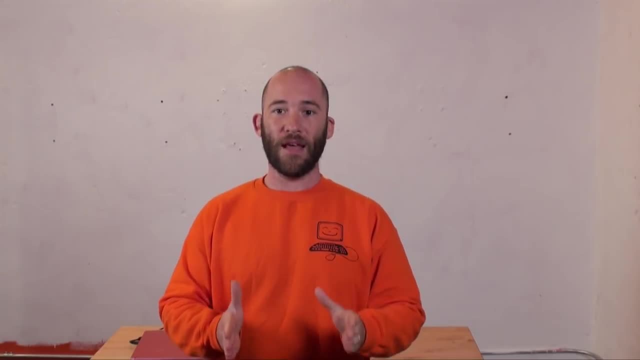 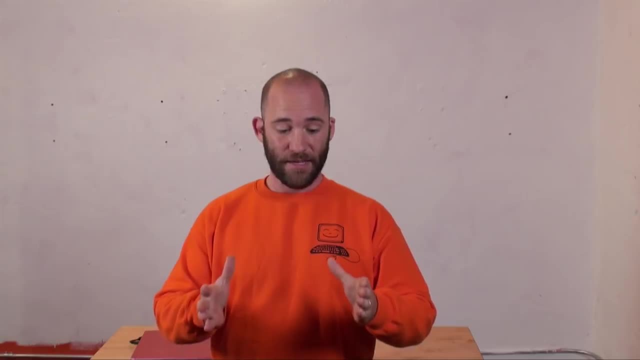 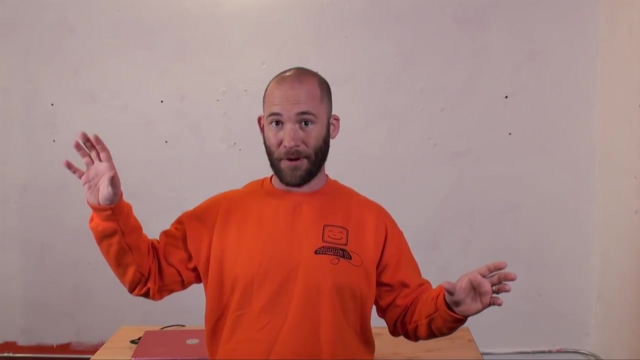 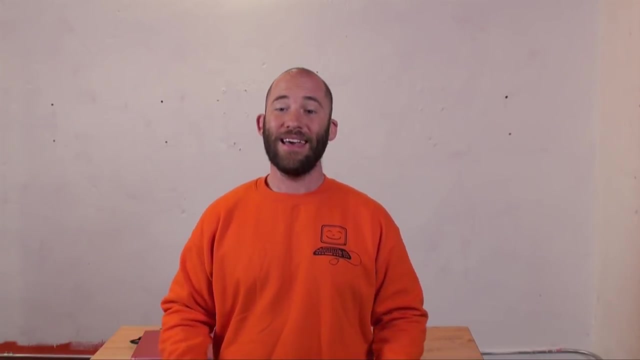 get to A print server on the network is a computer with a printer attached that can share out that printer to other computers on the network, So somebody can print, press, print on one computer and it will print out on another computer. A web server is simply. 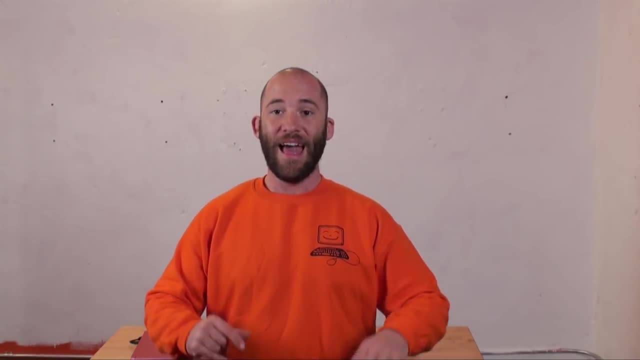 a computer with special software installed on it that allows that computer to present to people going to that computer. So all the server is is a computer on the network that provides services to other computers. Now this might be Windows 2008 server Windows. 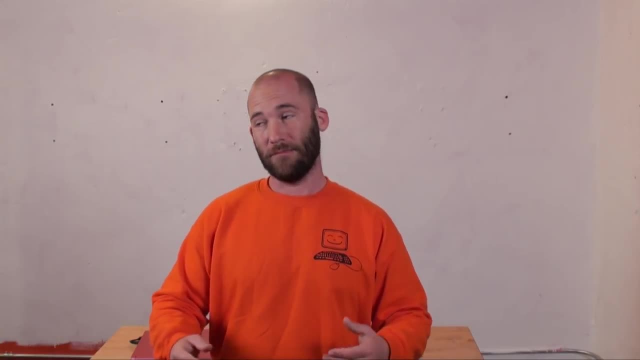 2003 server, Ubuntu server, Red Hat, Linux Enterprise Server Edition. It can be that, Or it can also be a Windows XP Home Edition computer that simply has a shared folder that everybody can access and grab files. So one of the big things that I want to get through. 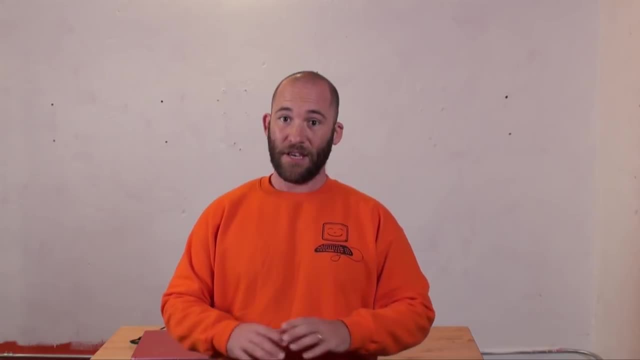 your head is that all the server is is a computer on the network that provides services to other computers on the network. Many people waste a lot of their own money and a lot of other people's money because when they go, oh I need a file server. 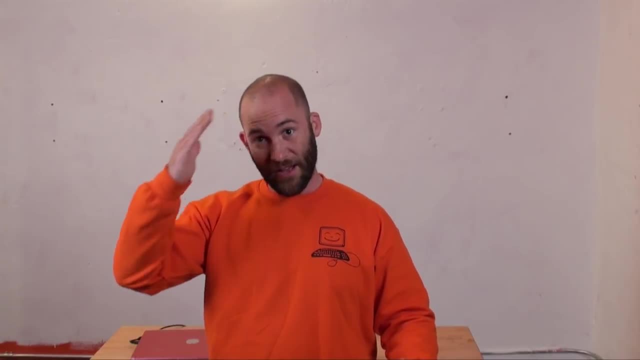 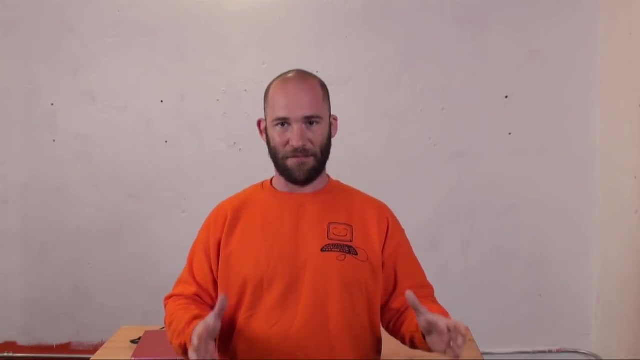 So let's say they have a little office and they have five people in that office and they go: oh, I need a file server. they run out and they spend $4,000 on an enterprise class Windows 2008 server And they can now share out the files to everybody in the office and 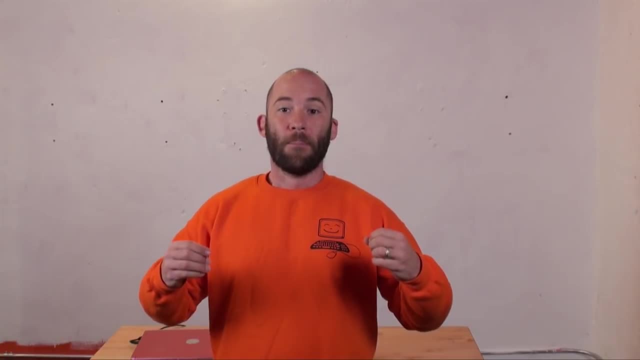 they go. Wow bonus: I now have a file server. Well, they did not need a full Windows 2008 server in order to share out a few files on the network that they could have used, Like I say, Windows XP Home Edition. 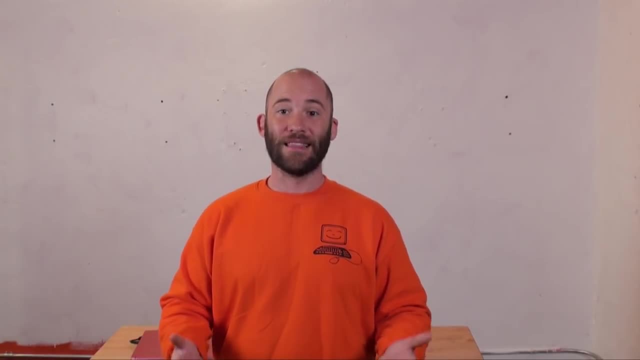 Home Edition to share out files in the network and it would have been a lot less expensive. So the main thing when we define server is that to be a server, the computer doesn't have to have server in the name of the operating system. All the computer does to have to be a server is it has to provide services to other computers. 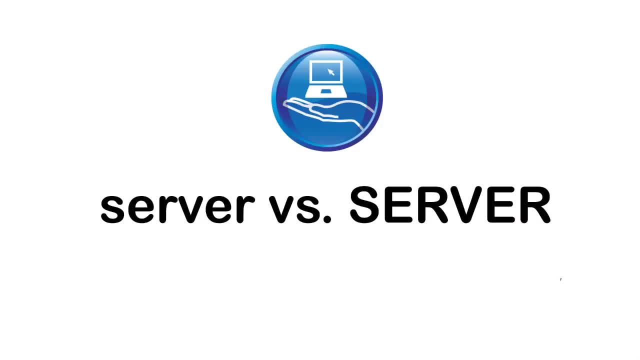 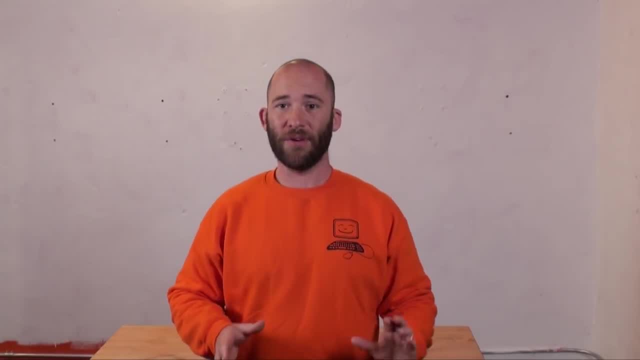 on the network. So now that we've defined what a server is, so a server is a computer on the network that provides services to clients on the network- We have to kind of differentiate between servers and servers. What do I mean by that? 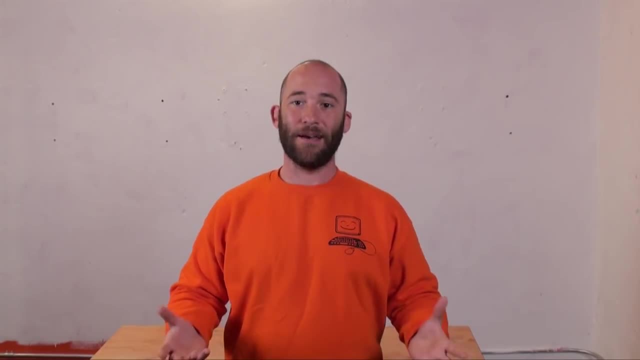 Well, in the real world you basically have two different types of servers. You have the little file server sitting in an office with five people that people either back up files to or they get something off of everyone Once in a while. it is a server, it is useful, people share information. but if the server 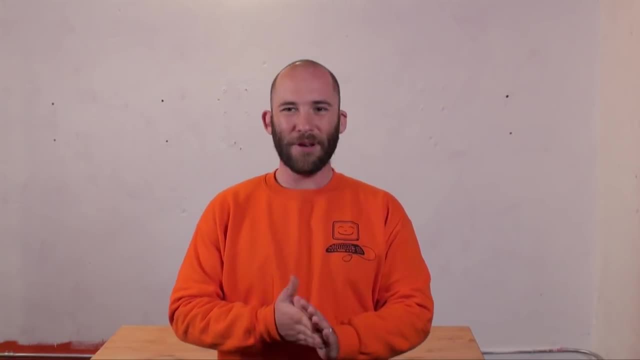 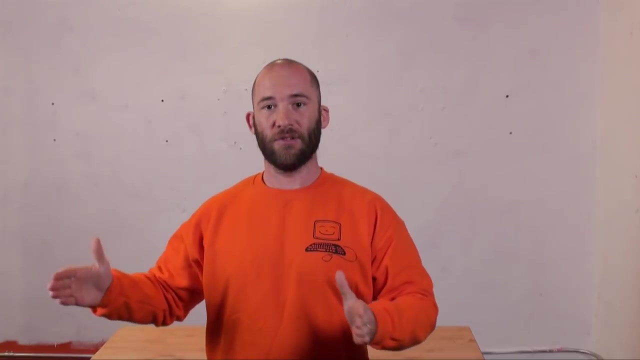 crashes or something goes a little hinky, nobody's really going to lose their mind over it. Nobody's going to get fired over it. Then you have servers- Servers- real servers are computers that have to be on 24 hours a day, seven days a. 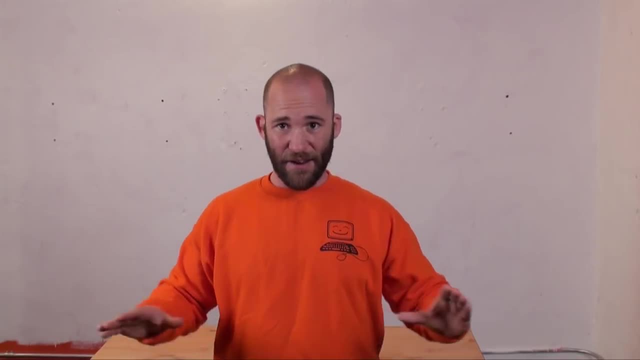 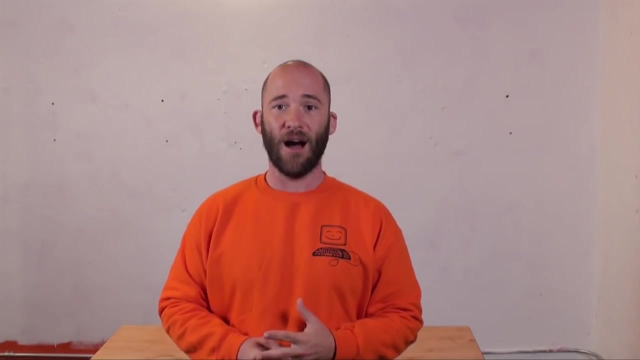 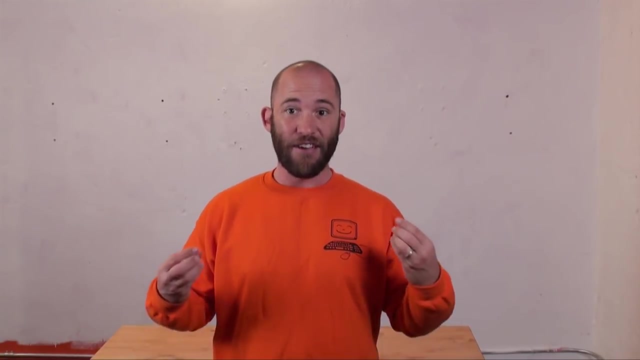 week, and if they stop functioning ever for any reason, everything just goes to absolute hell, Like with this company everymanitcom. our web servers, our media servers, have to be online 24 hours a day. They rarely even get rebooted. They get rebooted, maybe once a month, more likely once every two or three months. These things have to be rock solid, stable. If anything happens, they have to be able to survive small problems. so if there's a small problem in the operating system or the hardware, they have to be able to survive. 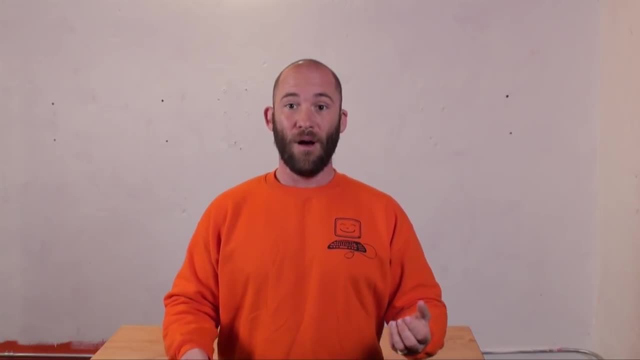 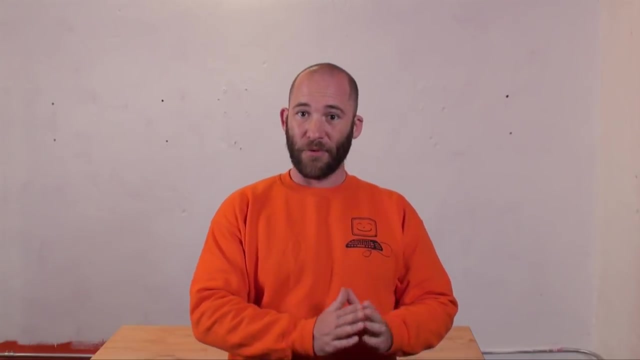 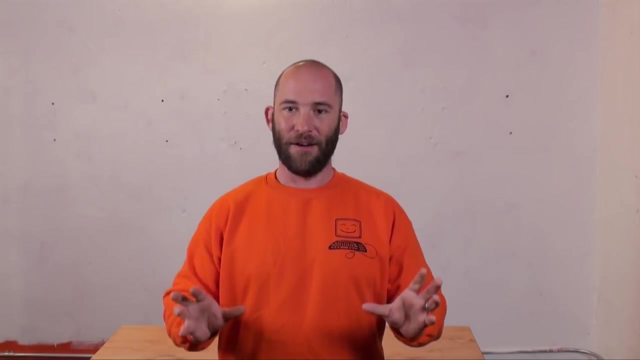 that and keep going, because if something fails, well then the entire business just goes away. We've defined server as providing services for clients on the network, but then what you have to think about is you do have two very, very different types of servers. 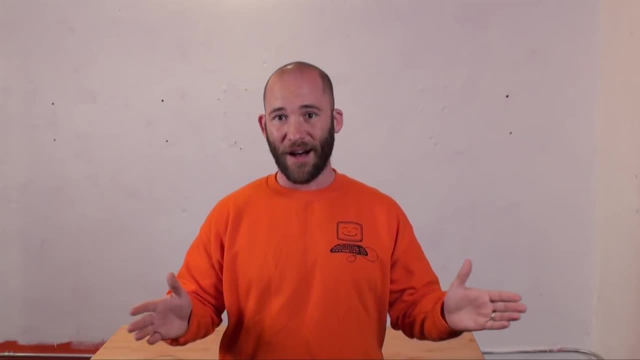 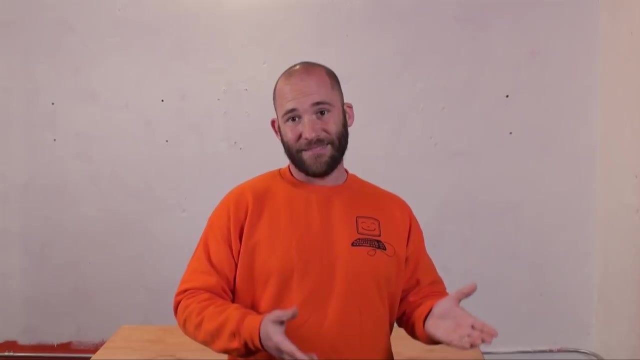 You have the server, like I say, that deals with five people in an office. It has a printer connected to it. It has some shared files. Again, Interesting dies. it's sad, you know we shed a tear or whatever, but but nobody's going to lose. 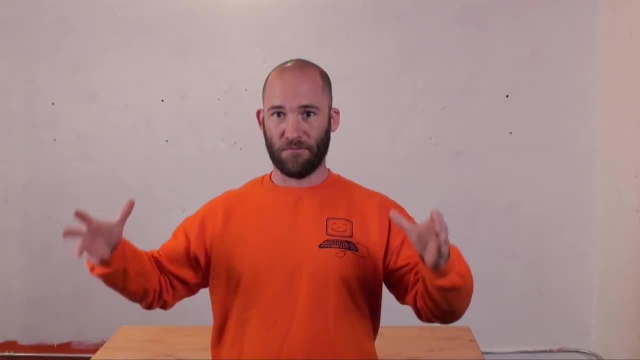 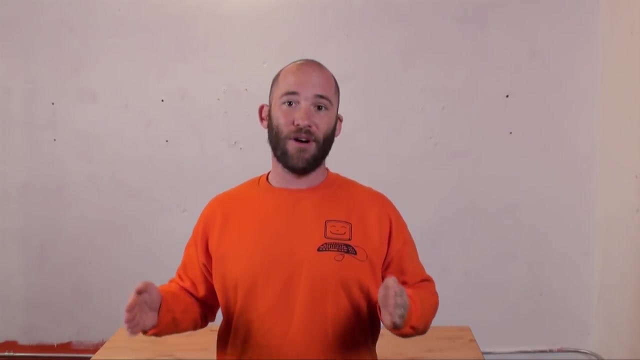 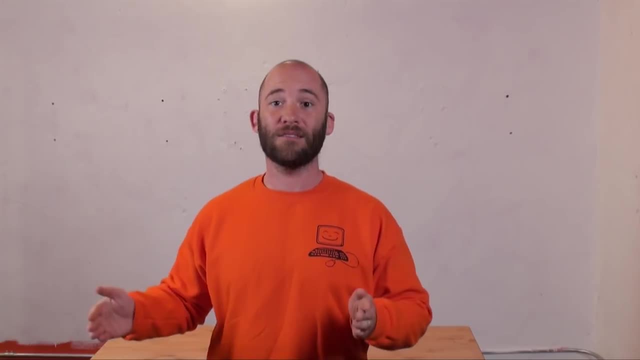 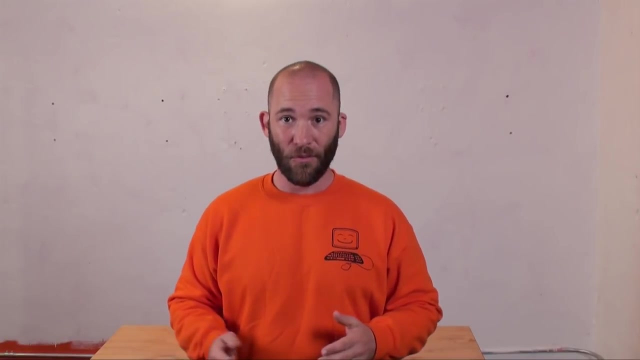 servers that they're going to talk, be talking about. they're going to be talking about rock-solid pieces of equipment that, basically, should never fail, so so just keep that in mind. there are two different types of servers in the world, and we're going to go into that in these next two sections, when we 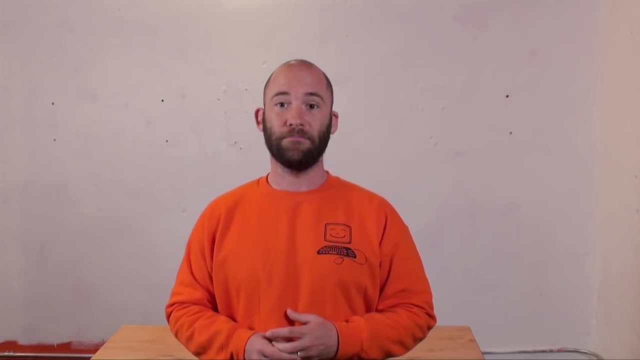 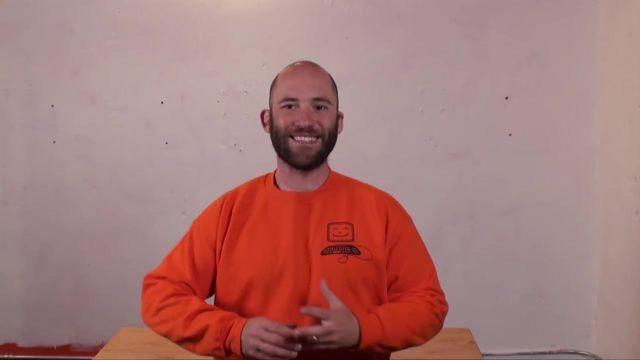 talk about the server operating systems and then server hardware. so let's take a moment to talk about server operating systems. as we said before, the little Windows XP home computer can be a server. you can play video games on it. but the issue with that little XP home computer is: 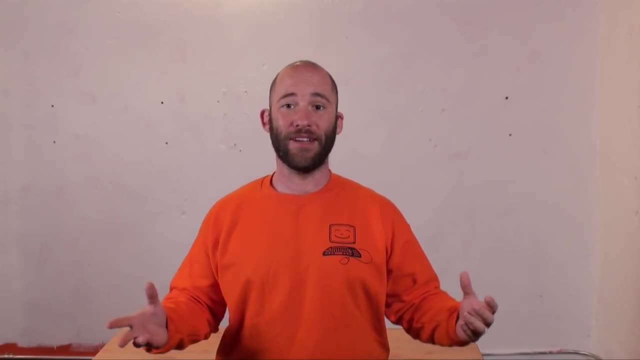 it's not designed to be on 24 hours a day, seven days a week, to never be rebooted, to never really need repairs. it's built to you know, to be a little computer. you can either do some word processing or play video games on. well, Microsoft and all the other companies out there, on top of creating desktop. 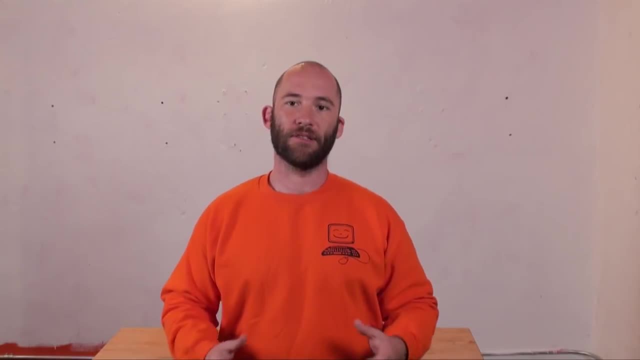 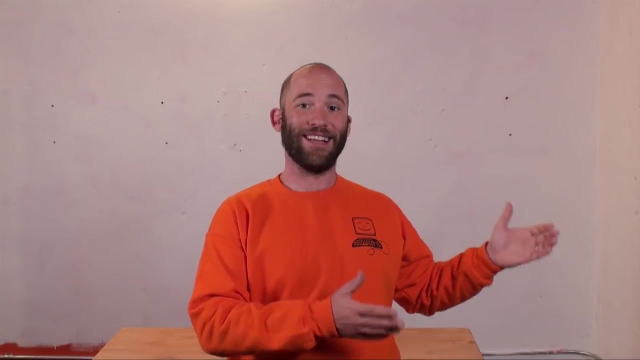 operating system operating systems they also create. server operating systems are more robust, more stable and generally more secure than the desktop operating systems. so if you're thinking, you know why don't I use that Windows XP home computer? because that's going to be a lot less expensive than buying a. 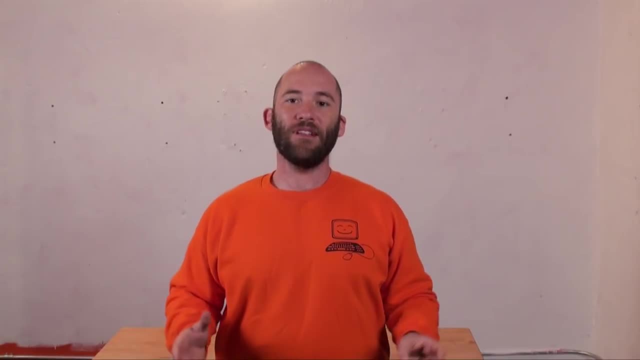 full-fledged Windows 2008 server. it really depends on what you need that server for. if you need to, you know, share files to five or ten people in an office, a little Windows XP computer would be fine for you. Windows 2008 servers or any servers, whether they're Linux or Mac OS actually. 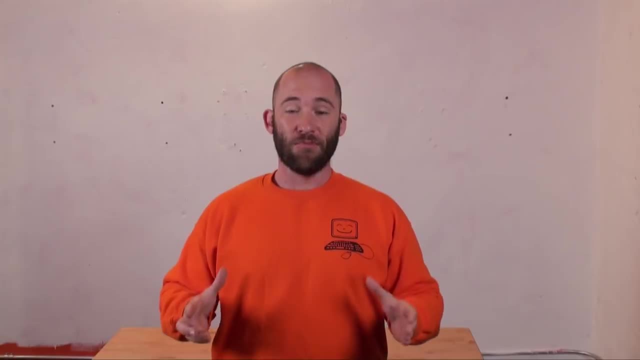 has a full server. they are made to be much more robust and to deal with many more incoming connections than than the little home desktop computers. imagine and realize that that real server operating systems, like if you're dealing with Windows 2008 server and you're using it for what's called an active 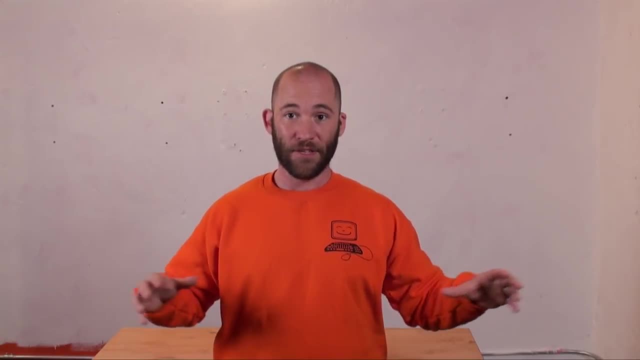 directory server so people actually log into it and they gain resources to the network. one single Windows 2008 server can support up to 10,000 users, so that that server software is much more robust and can deal with far more users and far more issues than the little desktop operating system will. so the reason 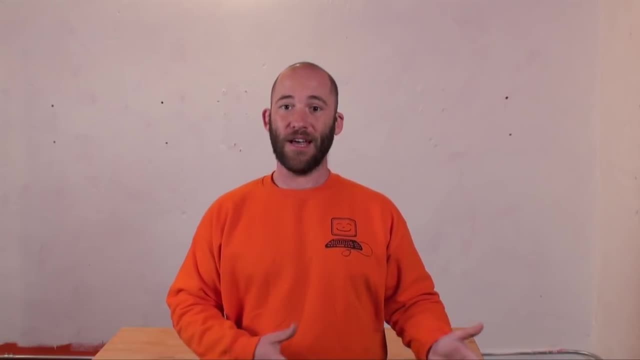 people use the- the server operating systems versus the desktop operating systems- is, again, they can scale up. they can deal with far more users that then a desktop computer can. one of the things that you have to realize when you're dealing with with server operating systems is: a lot of times they 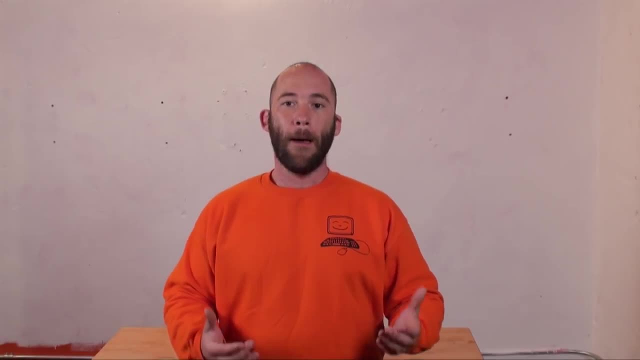 can seem much more complicated than desktop computers, because they actually don't come with as many of the the nice little friendly user tools that desktop computers come with. since you're new with servers, something to to think about is that every time you put a piece of software over the top of the desktop- custom software- you could get some very good results. you could get a very good result. 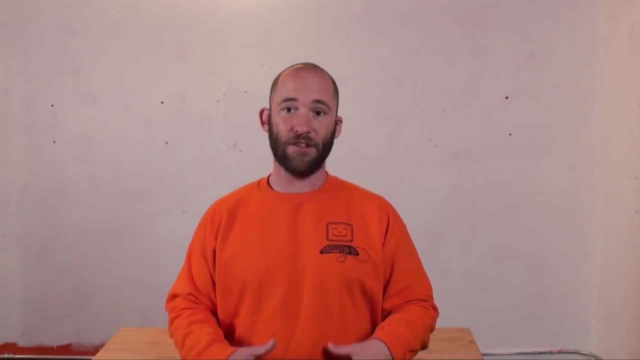 software or put a piece of functionality onto a computer, into the operating system, not only do you get that extra functionality, but you also get possible extra flaws, bugs and defects that hackers can use to compromise that system. so when you install flash onto your computer, you like it. 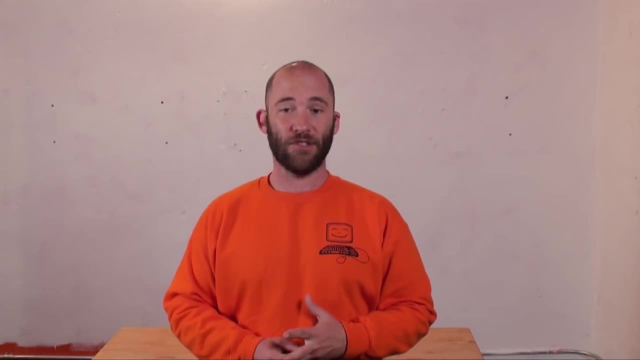 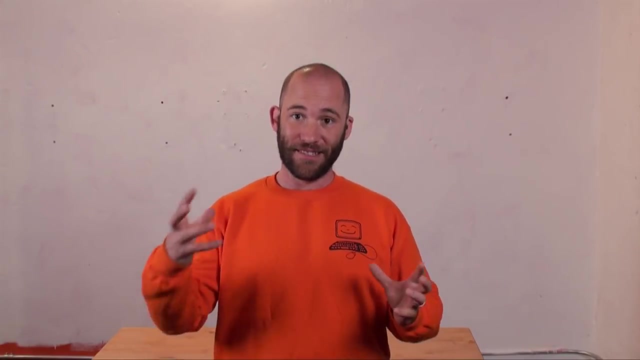 because you can. you can watch videos. you can watch this video because you have flash installed, but that flash actually has security holes that hackers can use to take over the computer. so when the vendors create server operating systems, they don't put in as many of those nice little. 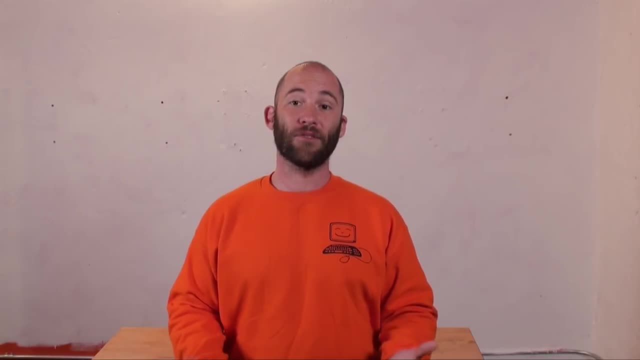 features into the server operating systems because they want to make the server operating systems more secure. so if you're dealing with a Windows 2008 server, when you go into it you're going to notice that it's it's much more difficult to get around and administer that server. then it is a. 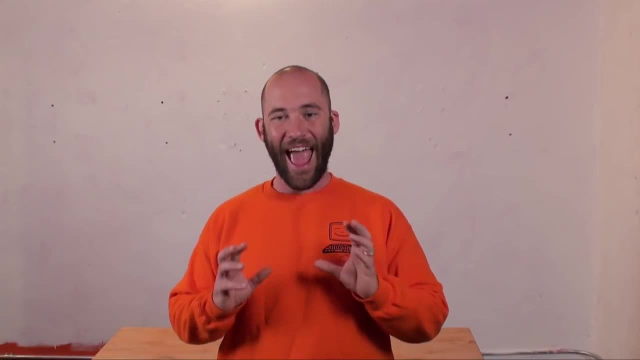 normal server. so you're going to notice that it's much more difficult to get around and administer Windows desktop computer because there's not as many nice fancy little flashy wizards and easy to do stuff. if you use Linux, like if you decide to use Ubuntu Linux as a server- you'll notice if you 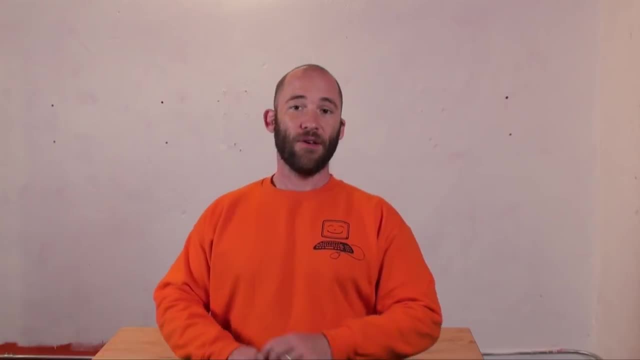 download and install the desktop version of Ubuntu Linux, you get a nice little graphical interface. you can go in, you can left-click, you can right-click and you can do all the stuff that you think of when you use a computer. if you download the server software after it reboots, you're going to be 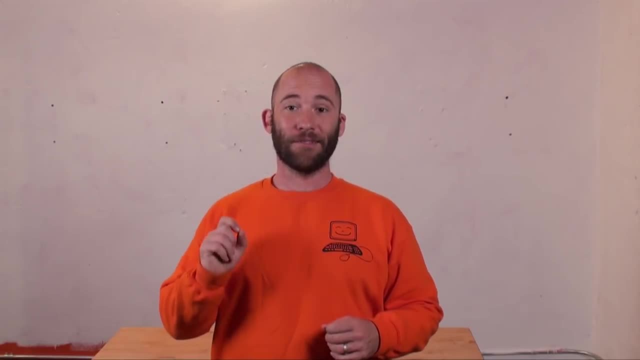 seeing something that looks like this. and you're going to be seeing something that looks like this, that looks like a DOS prompt and there's just gonna be a little cursor that's blinking at you and it will only do whatever it is you you type into it to tell it to do so. what, what, why they do. 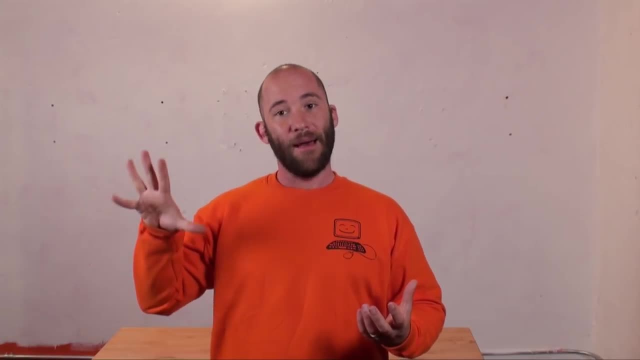 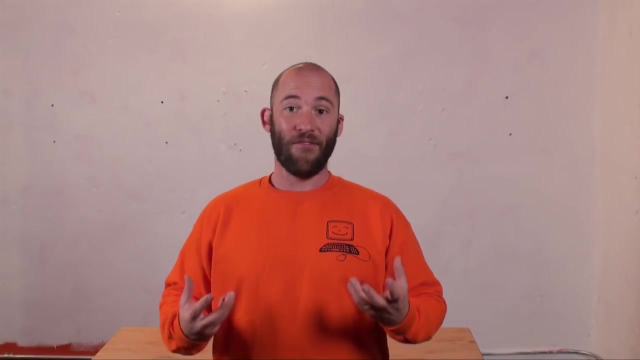 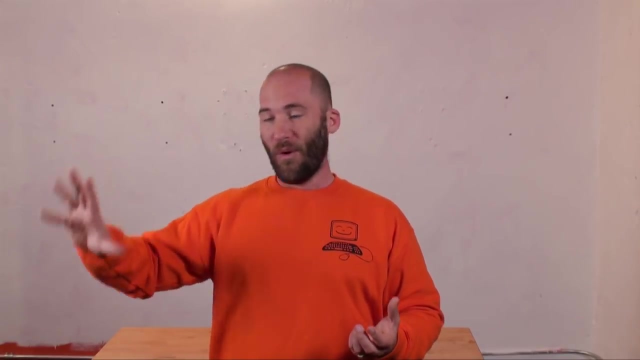 that is because all those fancy little graphics that that make the server easier to use also create security holes. so if you want a very secure Linux web server, you don't want all the graphical stuff. you don't want Firefox installed you, you don't even. you don't even want the the. 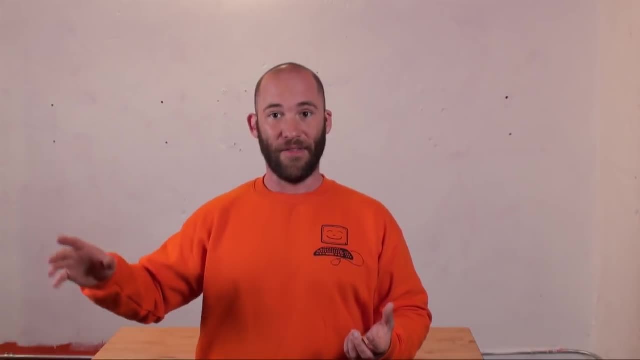 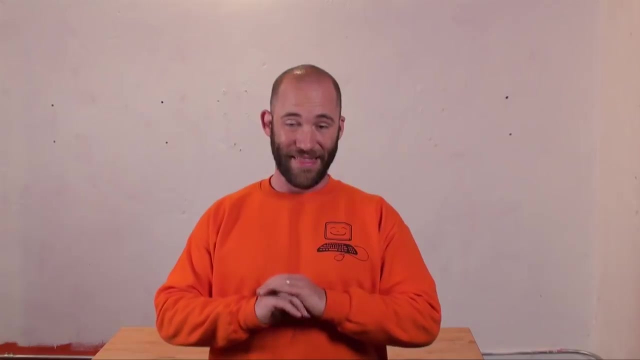 starting screen. but you do want the, the GUI. you don't want cursors and buttons and all that. you just want that little, that little DOS prompt so you can type in and tell it exactly what you want it to do, and that's, that's all it will do. so when you're dealing with the server operating systems, 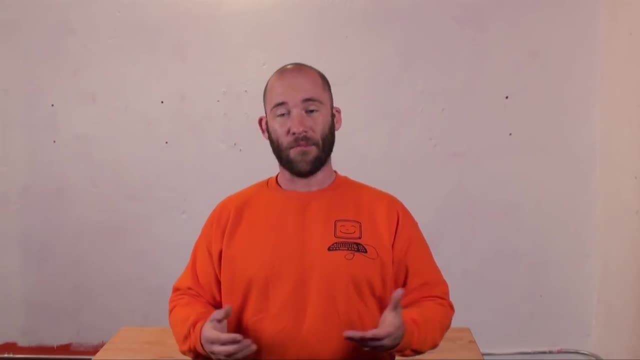 although in many ways they can be much more sophisticated or are much more sophisticated than the desktop computers and they're not necessarily as user friendly. so you really have to understand what you're doing before you you start going in there. it's just starting to with stuff, because if you do, if you do something stupid, it can be much more. 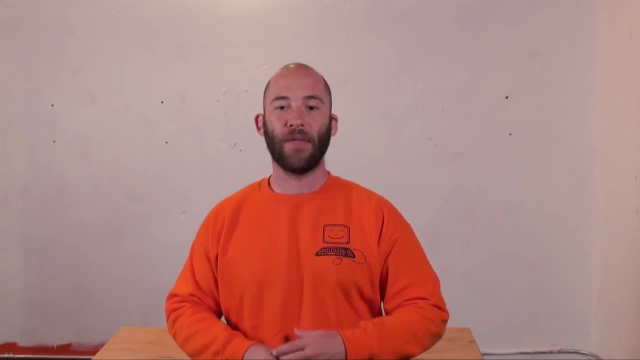 difficult to get back to where you came from the the last part, when you're dealing with server software. so we've talked about the server operating systems. server operating systems when you go to buy software, let's say backup software or utility software. one thing to just to realize, to know, is that software is going to be much more expensive than the normal comparable desktop versions. so, and when I had the repair shop, we used Acronis for our backup solution, whether it was desktop computers or servers. well, the the Acronis for a desktop computer was anywhere between fifty to a hundred. dollars, depending on what what edition. we bought the backup software for the servers that we install. it seems like it's the exact same thing, but for whatever reason that was six to seven hundred dollars. so this is something that we're going to be using for the rest of the software that we're going to be. 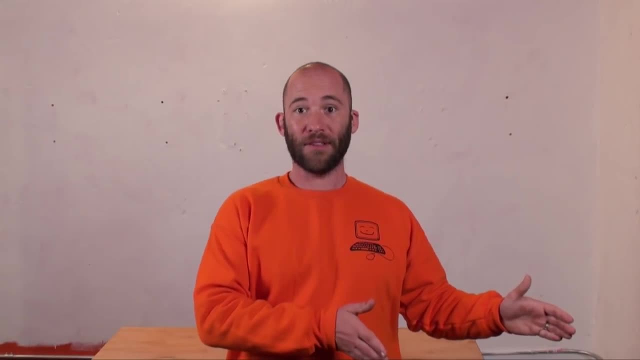 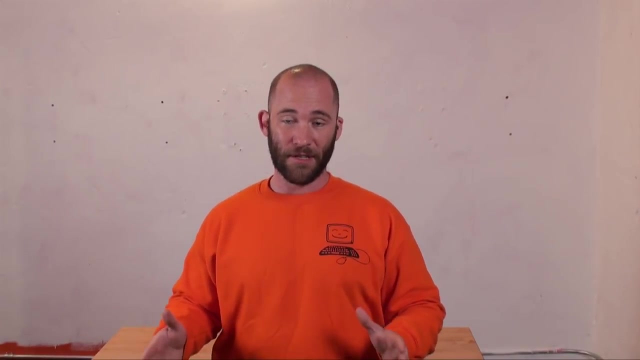 using for the rest of the software that we're going to be using. for the rest thing, to realize, when you're deciding between using a desktop operating system as a server or a server operating system as a server, is the software for that server operating system is going to be more expensive. again, we used a disk. management. you know it's partitioning software to enlarge or shrink partitions on a desktop computer it cost $50. for a server it cost $600. basically the same functionality. one was for a server, one was for desktop computer- ten times the cost. so we've kind of talked about the server operating systems. remember any computer? 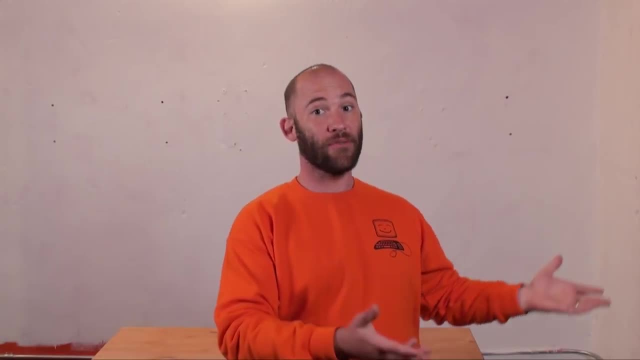 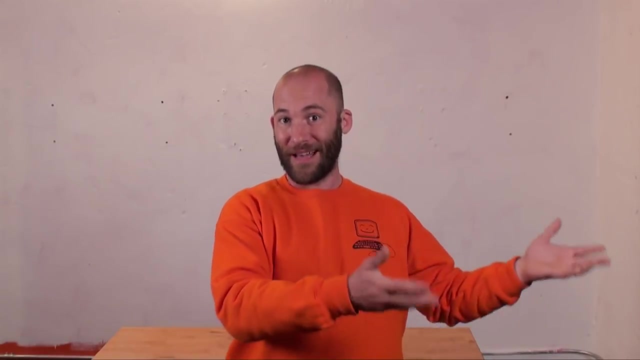 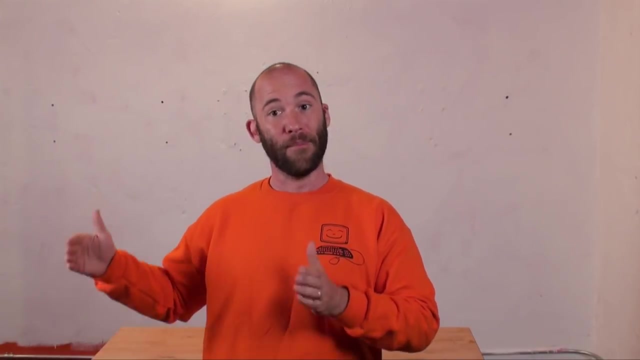 that provides a service on the network is technically a server. but then you have two types of servers. the server that supports five users- you know it's it's low computer, has a couple files on it, has a printer, and those servers. servers support up to 10,000 users at a time are much more robust, are expected. 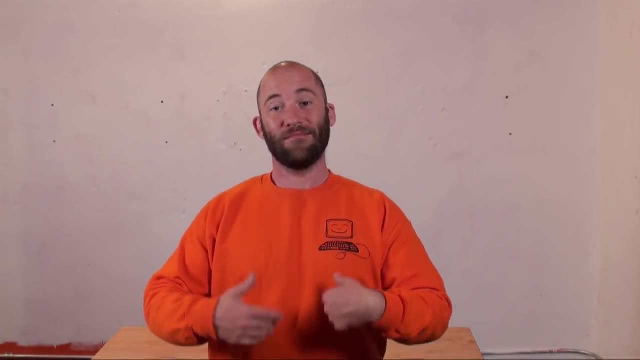 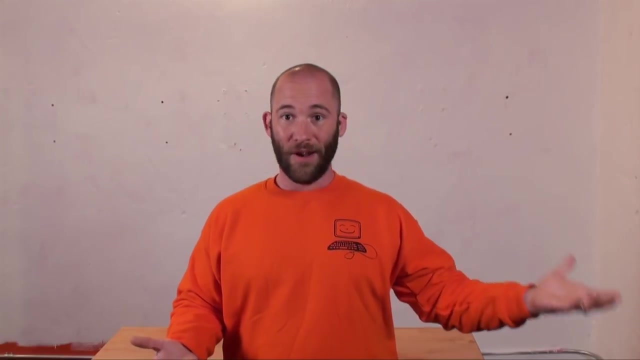 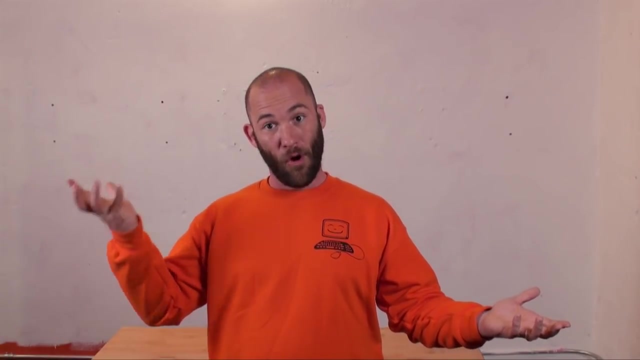 to never be rebooted, etc. when you're looking to install a server for yourself or your client, really think about what you need because, again, like I say, that a little Windows XP computer is fine for five people and is very inexpensive. the server- that Windows 2008 server- is very robust but very expensive. like I say, 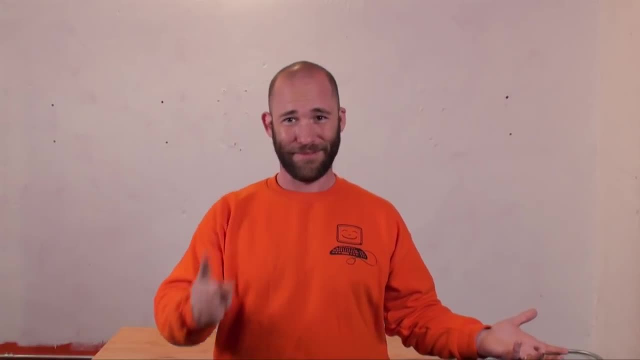 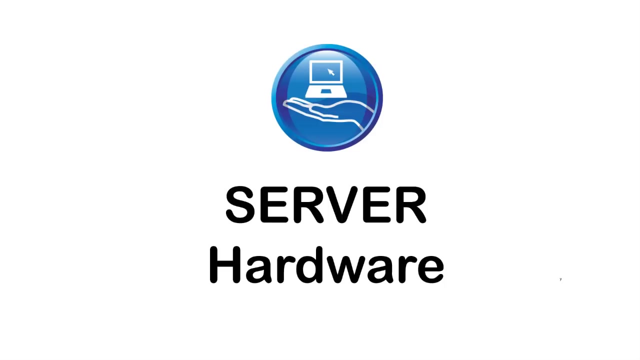 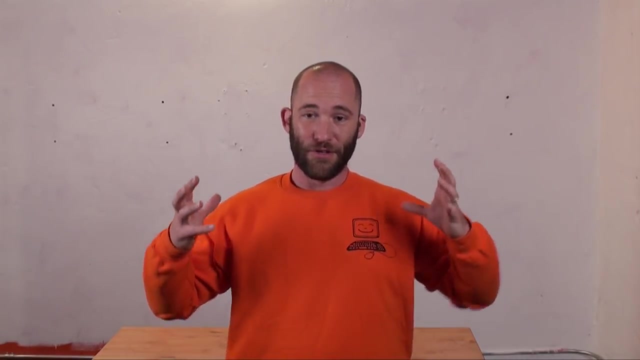 even the backup software was $600, just just for one piece of software. so that that's a brief introduction on that, on what server operating systems are. now let's go into and we're going to talk about server hardware. so we just talked about server operating systems. so so server operating systems. 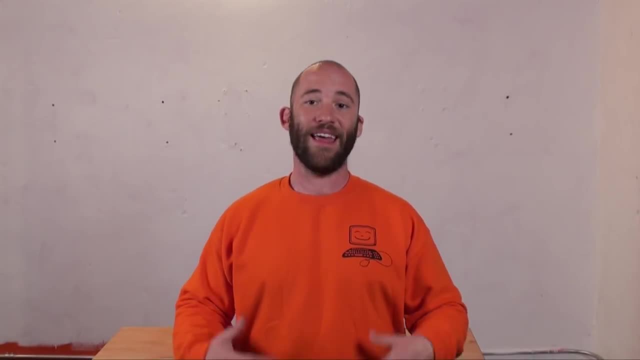 Windows 2008 server, Ubuntu server edition, anything like that. those are operating systems that are built to be on servers that are going to be very robust, very tough, more secure, etc. well, the same is true of server hardware. so you can use any hardware to create a server. you can go out to Best Buy and you can buy the crappiest little. 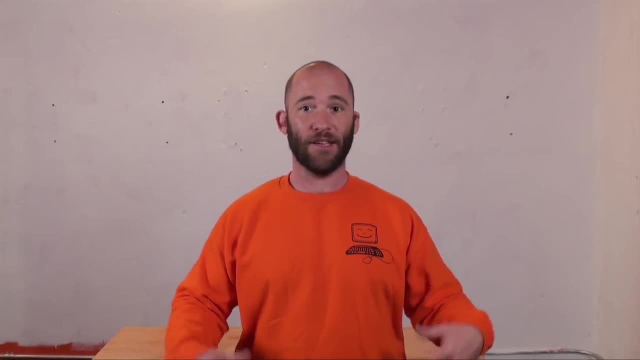 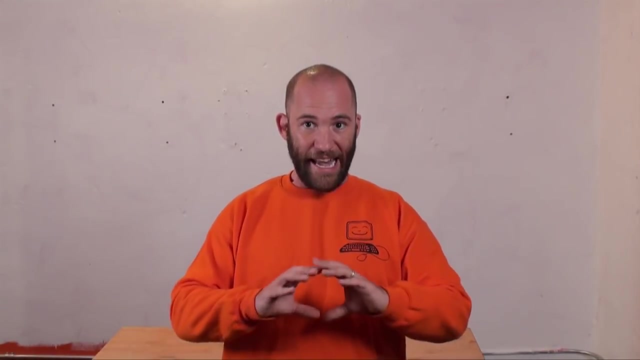 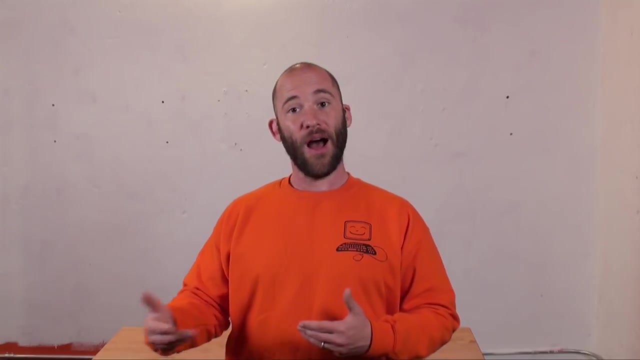 machine. you can throw it on the network and you can share out files and you can use that fine as a file server or whatever type of server you need. you don't need need specialized hardware for servers but just like with the server operating systems, they do make special hardware for servers and and if you need, 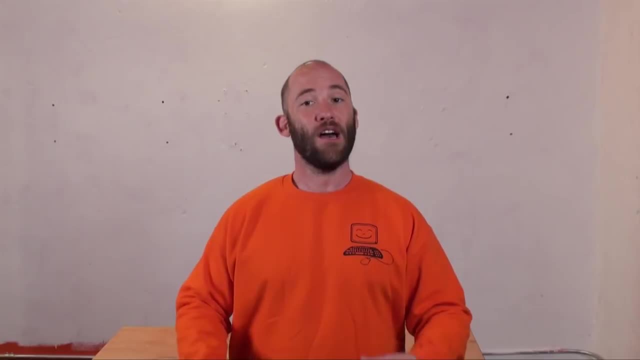 your server to be up 24 hours a day, seven days a week, etc. you should really think about using real server hardware, the the. the first piece of server hardware that you probably know is is server processors, so in Intel these are called Xeon processors. basically the reason. 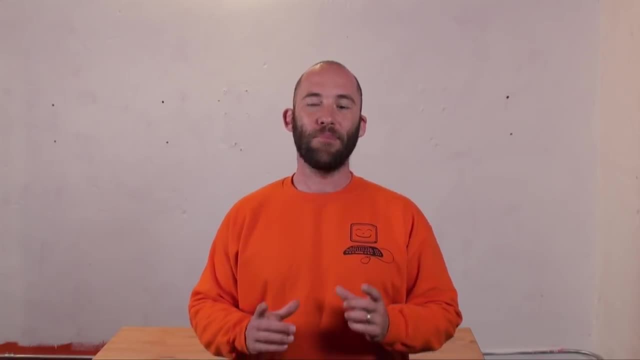 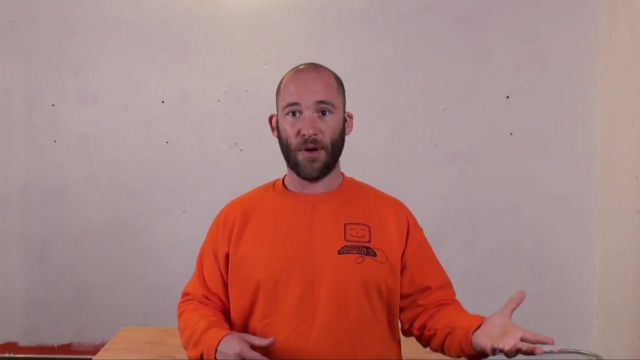 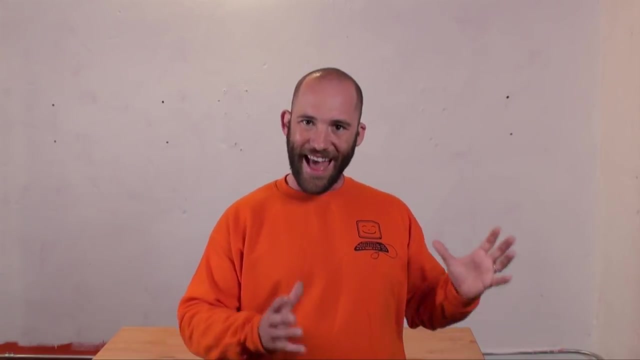 you want to use a Xeon processor is that processor is built for dealing with the tasks that servers normally deal with. so if you want a really fast video game machine right now, you probably buy an Intel i7 quad-core processor and that is built for video games. that will be very good for video games. well, what you need 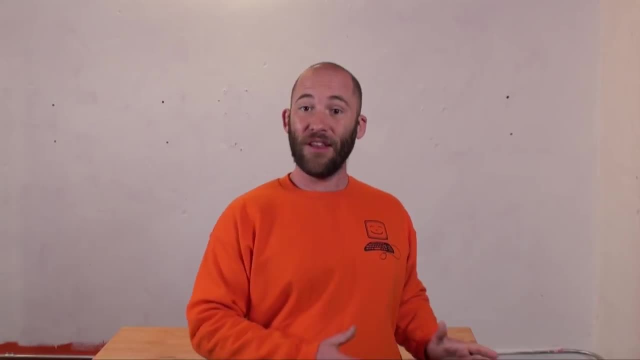 in a server computer is not the same as what you need in a video game computer. so you would go out and you would buy a Xeon processor. these processors just are. you're very good at just chugging through and just dealing with data and doing the stuff that that server is doing. so the first thing is the Xeon. 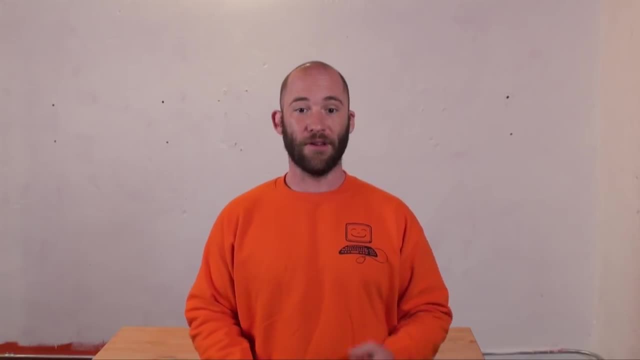 processor. again, you don't need to buy a Xeon processor to use a Xeon processor. don't need it. but it is better if you have a SPF. if you're using a server. the next thing when you're dealing with a server is something called redundant. 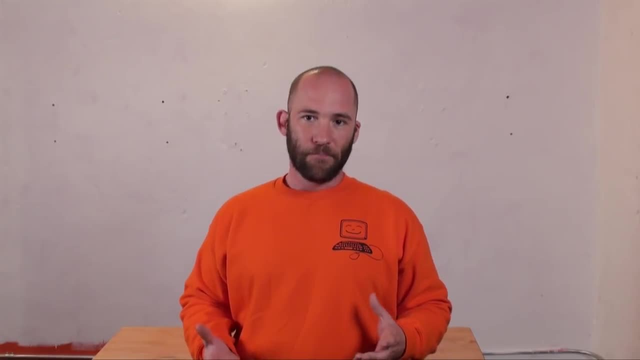 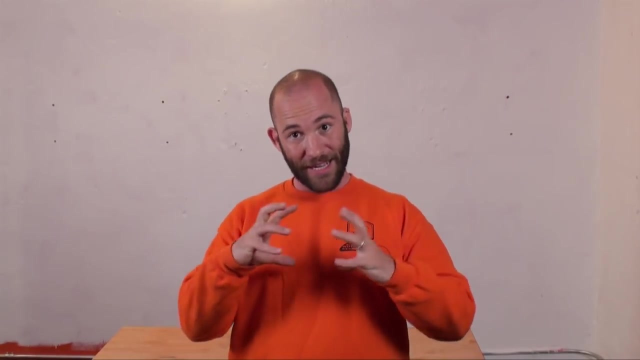 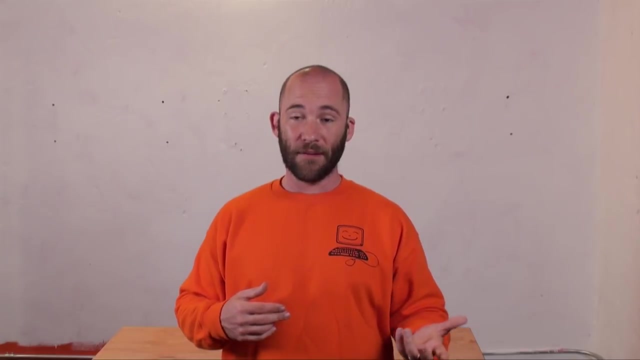 power supplies. so what the redundant power supplies are is within the normal form factor for power supply. they can fit anywhere between two to three power supplies in there, and so if one of the power supplies fails, the other two are still active and the computer stays on. so imagine if dust gets blown in or just 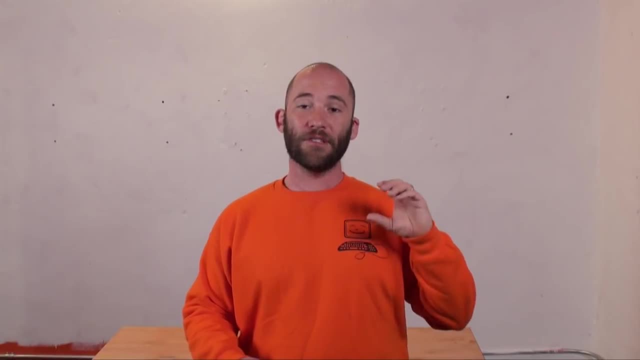 a capacitor or something like that and you're dealing with a server and you're blowing out any of the normal stuff. if one of those power supplies dies, the computer is still on. it's completely, still functional. most of these redundant power supplies are hot swappable, so you can actually, if one of those power, the 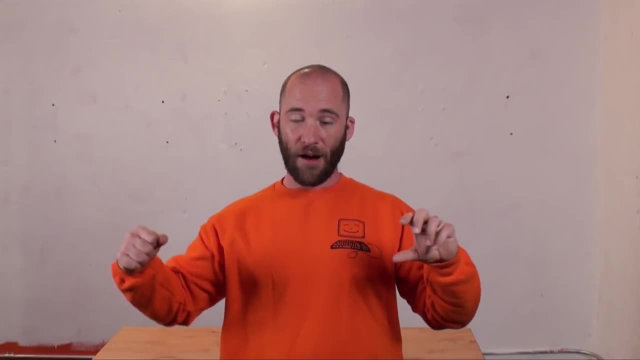 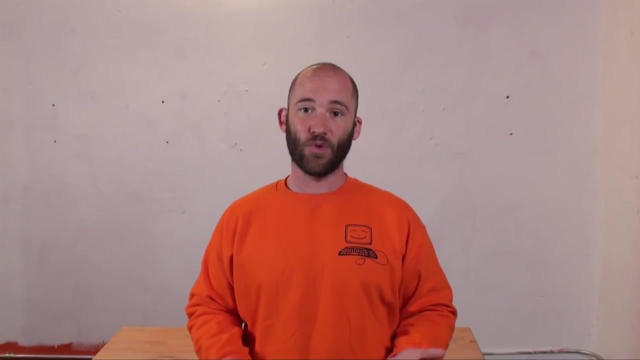 the redundant power supplies fails, you can pull it out, you can order a new one and just plug it in and go on your way. you do not have to reboot the system. that's that's hot swappable. again, almost all of these redundant power supplies are hot swappable, so with the redundant power supplies you can have anywhere, between two to three power supplies and then you can. you can be at the top of the different power modules and normally you can have anywhere between two to three modules. so you can. you can have up to basically, two power supplies fail. so that's what the redundant power supplies do, is they allow one power supply to. 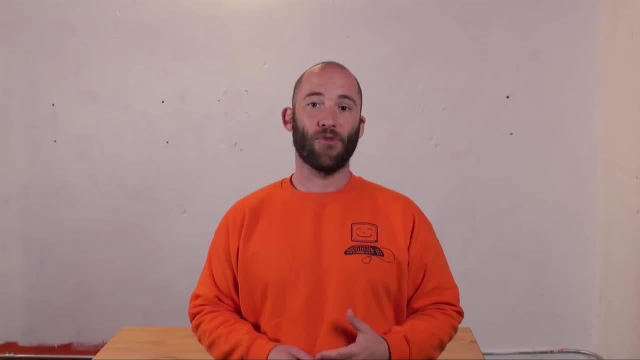 fail, but the computer stays on with the power supplies in most servers. you will also hear of something called RAID. RAID is a redundant array of inexpensive disks. Intro to RAID if you want to take a look at it. Basically, what RAID does is it allows you to 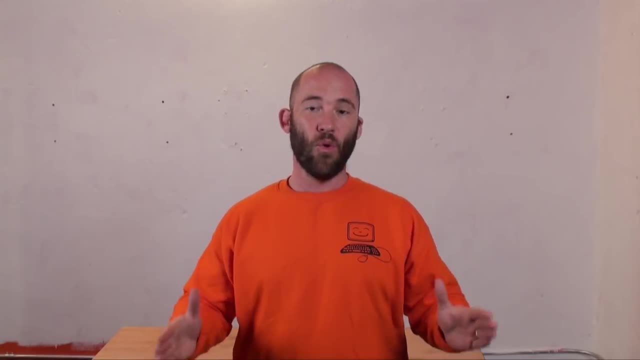 combine multiple physical disks into one logical disk. So most of the time if you have a server, you'll either have something called disk striping with parity or disk mirroring. Disk mirroring is where you have two hard drives in the machine that are identical, So one piece of data gets put on. 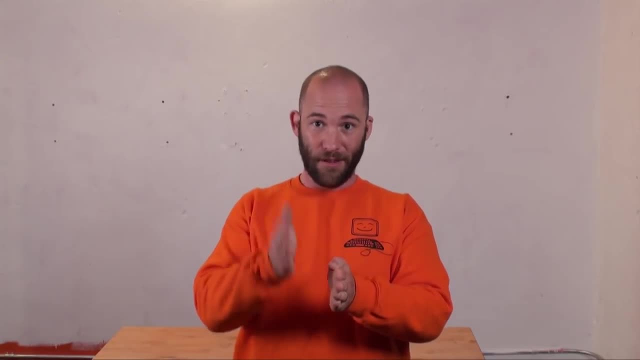 one. one piece of data gets put on the other. Another piece of data gets put on one. another piece of data gets put on the other. If one of these hard drives fails, the computer stays running because you have two identical hard drives. These hard drives are again what is called hot. 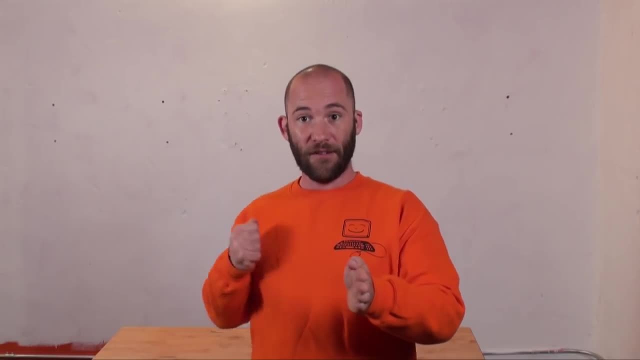 swappable. So if one hard drive fails, you pull out the drive that failed, you plug in a brand new hard drive. it does something. the computer does something called it rebuilds the array and then you go back to being redundant. So if one hard drive fails, the computer stays up. 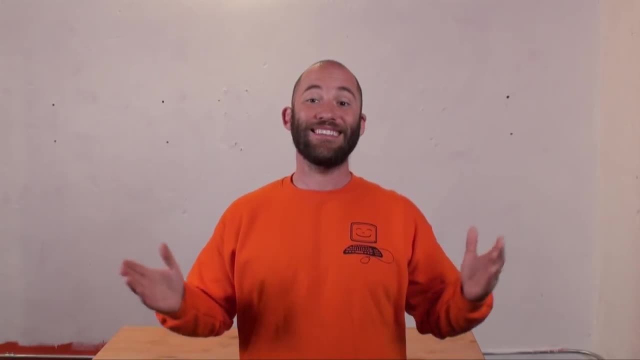 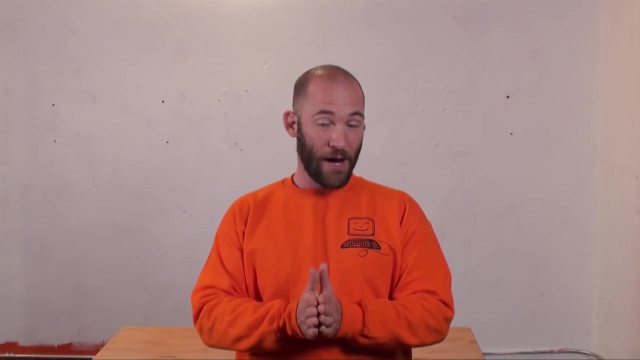 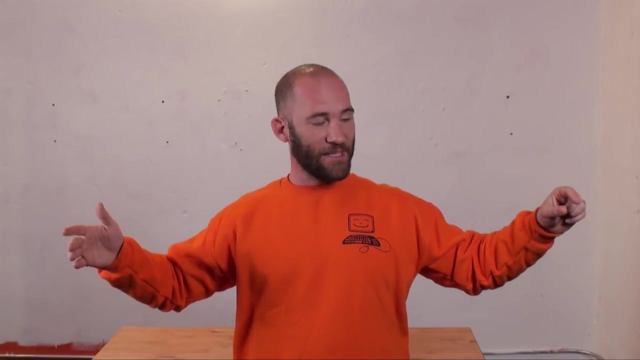 you pull out the bad hard drive, You put the new hard drive in, everything stays running. You never turn the computer off. This is all while the computer is still on. RAID 5 is where you can combine anywhere between three to 32 disks into one logical hard drive, And what happens is it stripes the data across all the 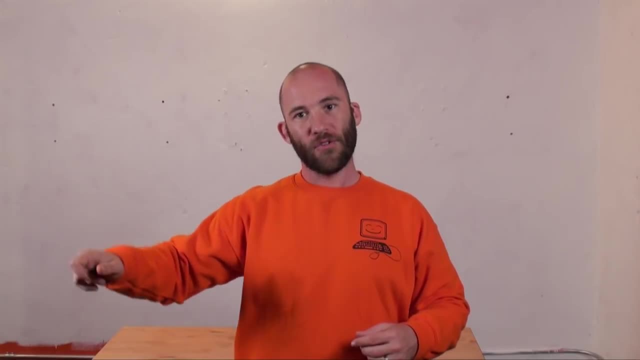 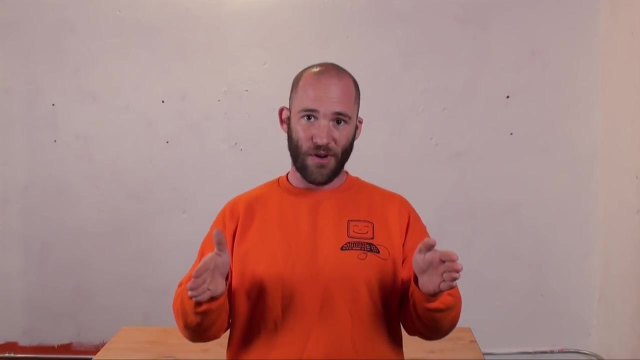 hard drives that you have in that RAID And then it has one hard drive that's used for parity. Basically, to make this easy, if you have five hard drives, it strikes the data along all those hard drives and uses one of the hard drives. It's kind of like. a recovery drive. So if any single hard drive in that RAID fails, you can pull that bad hard drive out. The computer still stays functional. You put the new hard drive in. it does something called rebuilding the array and you just go on your life. The computer or the server never. 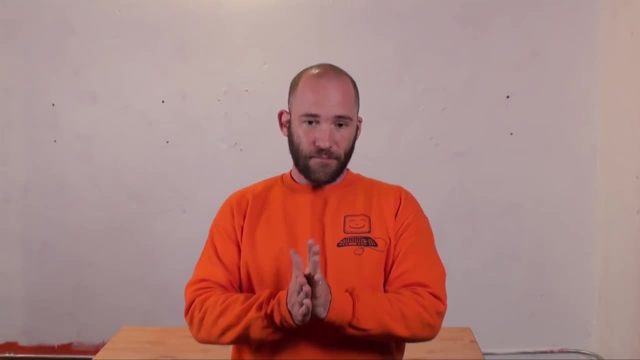 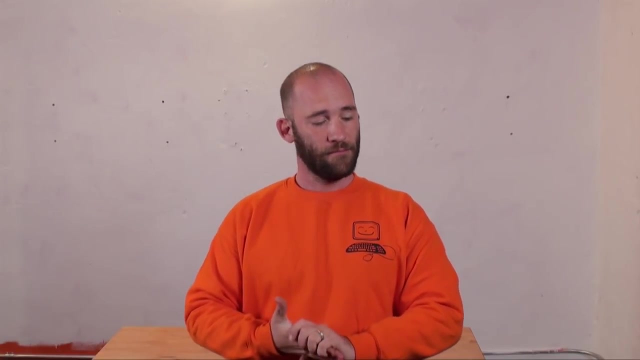 shuts down. So this is RAID. The last thing that you see in servers is it's called ECC RAM. This is error checking something, RAM. What this is is most RAM that you put into your computer like into a normal desktop computer and, frankly, what I put in my servers- ECC RAM- is incredibly expensive and I don't see the purpose. 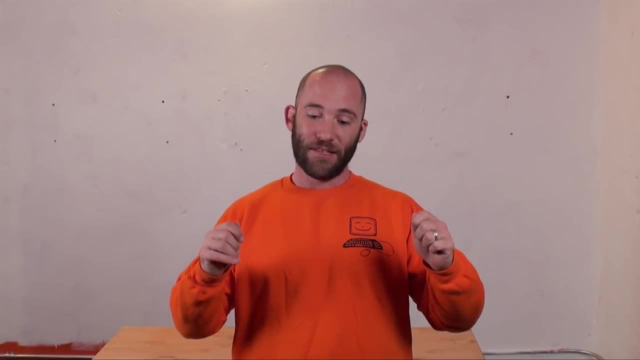 but we're going to tell you about it. What this does is when you normally boot up your computer, your computer normally boots up and it just accepts the RAM that's in there for what it is and you go on with your life. ECC RAM actually runs a check. 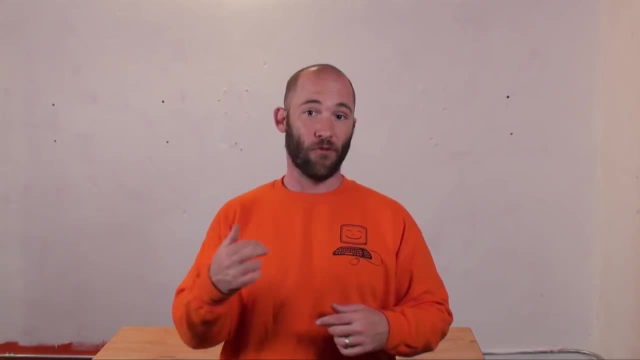 It runs a self-test of that RAM to make sure that the RAM is functioning properly and if it's not, it does a couple of corrections. This means that you don't have to worry about having any bad RAM, because bad RAM if you're using a desktop computer, if you're just doing, you know, PowerPoint presentations. 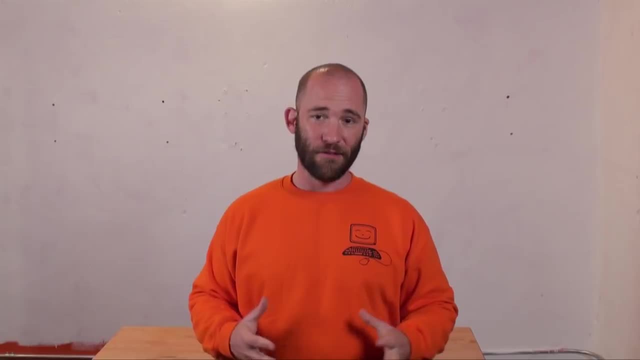 in Word. it's probably never going to affect you, But remember real servers that are that you know have a thousand. you know if you have a web server that has a thousand visitors an hour or if you know something that's really crunching a lot of information, if you have. 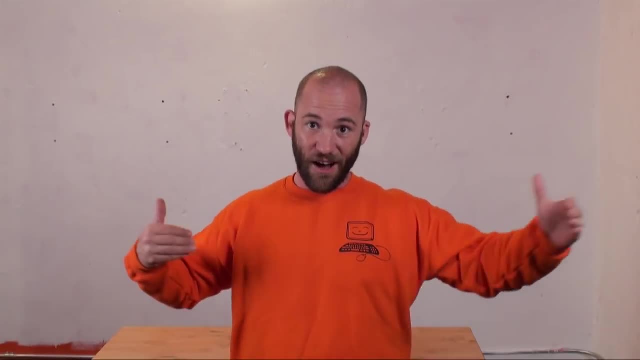 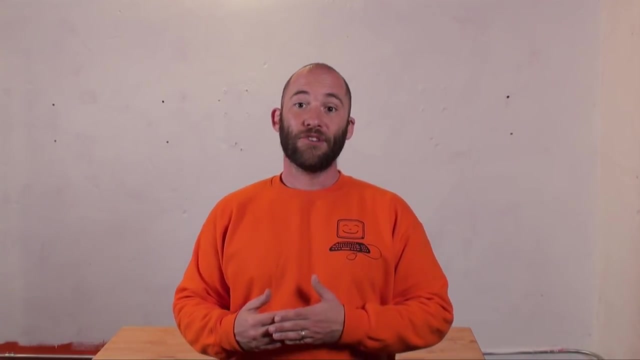 anything bad. really, it can start to cause massive consequences. You know, a little snowball turns into a big boulder. So the error checking RAM makes sure that the RAM is perfect and if it's not, it does some little corrections in there to make sure that it won't. affect the server when it's online. Again, this is nice because it makes sure you're RAM is perfect. It makes sure you don't have any small problems that snowball into bigger problems, but you're going to spend three to four times as much on your RAM when you. 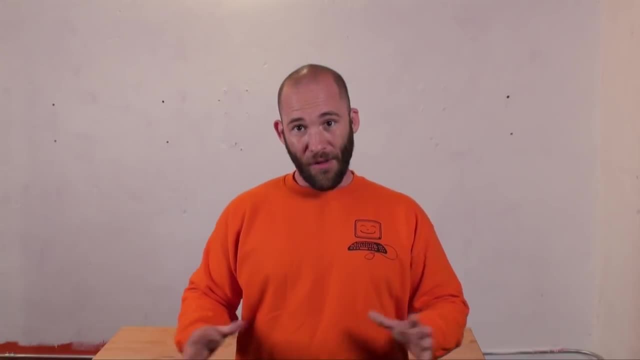 decide to use it. ECC RAM, out of all this stuff, is the thing I am least worried about. None of my servers use it. You know, maybe when I'm, maybe when everymanitcom has has thousands and thousands and thousands of people hitting it per hour, we'll worry about it, but this is something that 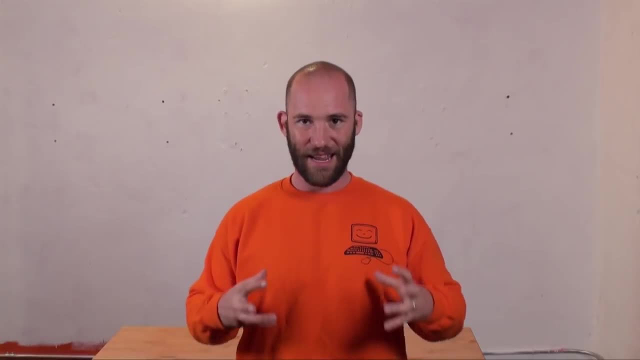 realistically unless, unless you really need really just a perfect, perfect system, you don't need ECC RAM. So we talked about the Xeon processors. These are basically just processors designed for servers, for server applications. We've talked about the redundant power supplies, So the redundant power. 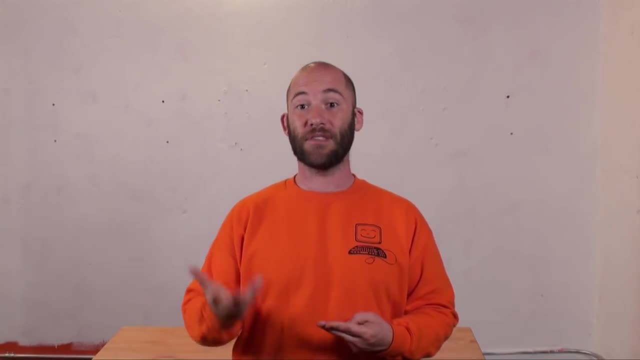 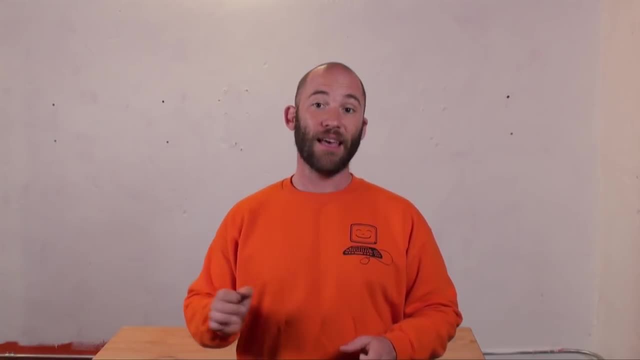 multiple physical disks into one logical disk. If any one of those hard drives fails, you can pull out the hard drive, put a new one in and the computer does something called rebuilding the array and just basically fixes it. We have an entire class on RAID called Intro to RAID. if you 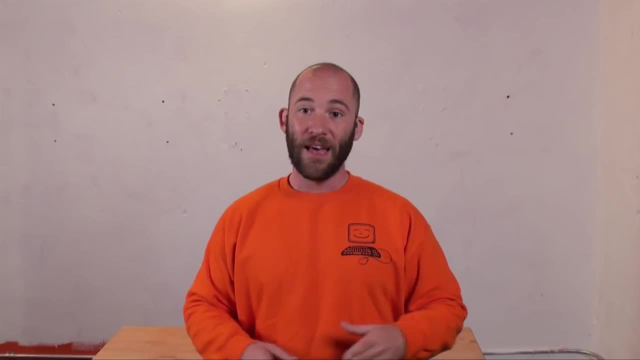 want to learn more about RAID. And then, finally, we talked about ECC, RAM. Again, this is RAM that does a self-test of itself and corrects problems if there are problems. Very, very good if you need the absolute most robust server in the world. And then, finally, we talked about RAM. So we talked about 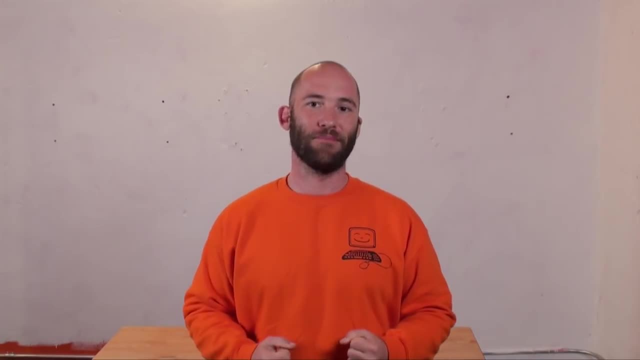 the world, but again it's going to cost you a foolish amount of money. I don't use it, but it's kind of your decision on that ECC RAM. So now that we've talked about what a server is, you know defining different types of. 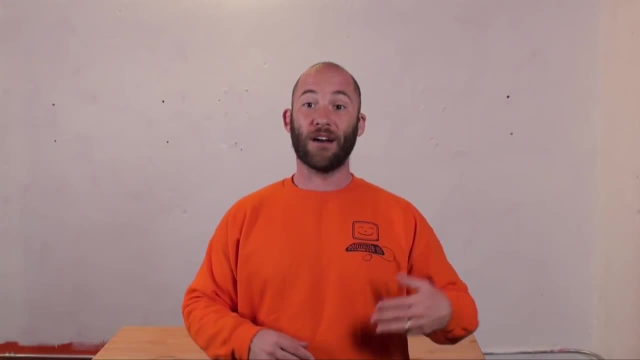 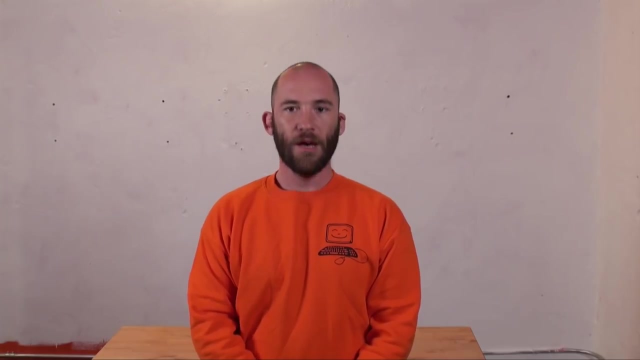 servers, the little server and the server. we've talked about the server operating systems and the hardware. now let's go into talking about the different types of servers. What do you use servers for? So now that we've gone over the basics of what servers are, let's start talking about 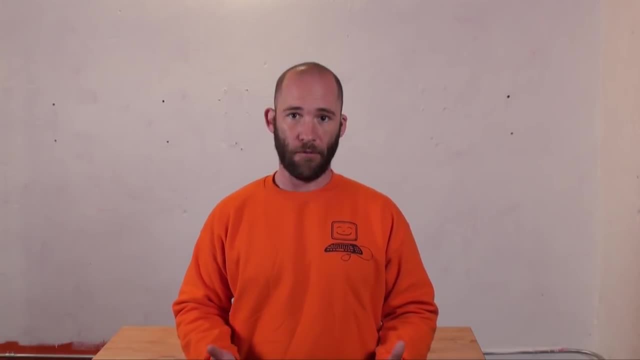 what servers actually do for you, What do they do for the network? The first thing that you have to realize when we start talking about all these possible functions of servers, whether it's file server, FTP server, web server, database server, terminal. 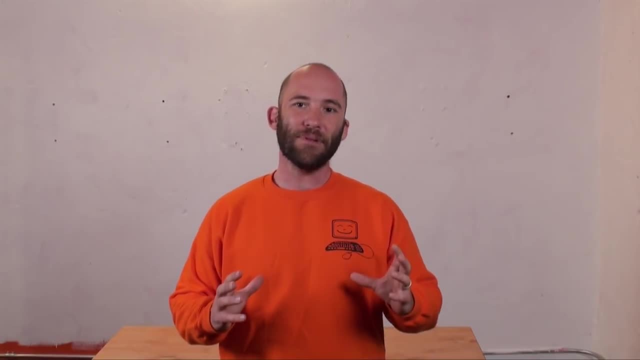 services, server, mail server et cetera is. these are simply server pieces of software, just like Word or Excel or PowerPoint on your computer. So one server, one physical computer with one server operating system can provide multiple server functions. So don't think that one computer can only do one thing. 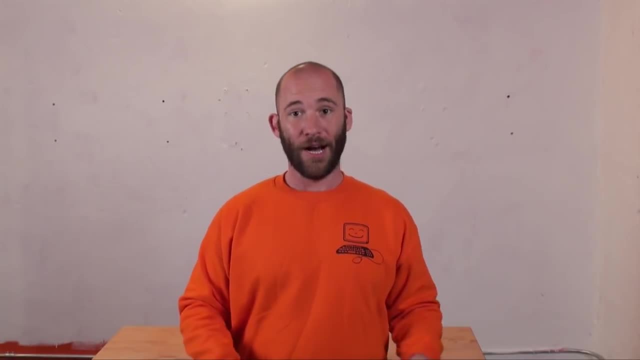 It's like your desktop computer. You know, your desktop computer can have Photoshop and Word and Firefox and all these other things. A server can be a mail server and an FTP server and an Active Directory server. It can be anything. It can be a web server and an Active Directory server all at one time. 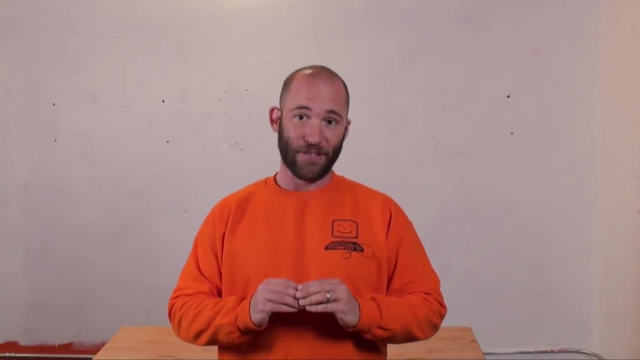 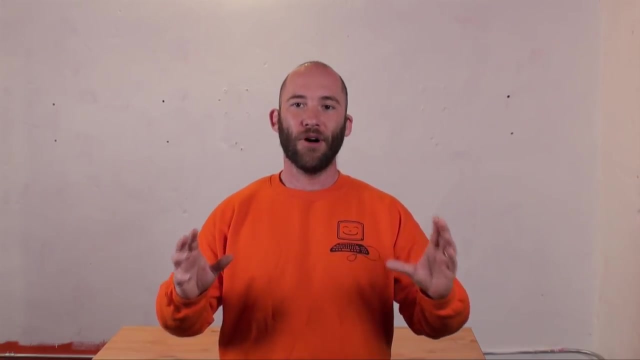 In this next little bit I'm going to break down all these separate server services into their own parts and talk about what these individual components can do. But I don't want you to think that you have to have a physical computer for each one of. 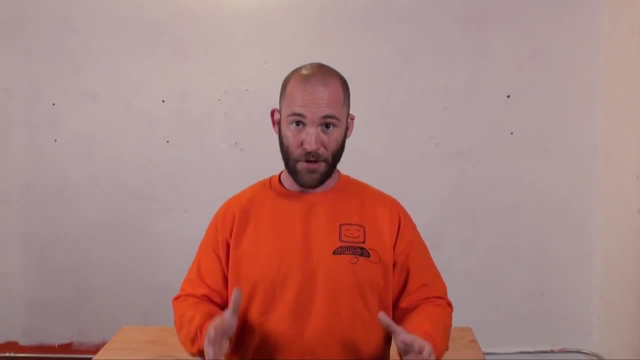 these components. They can all be on one computer- Windows. when you buy a Windows 2008 server, most of this functionality is already built. It is already built into it. So these pieces of software are already built into and included in the operating system. 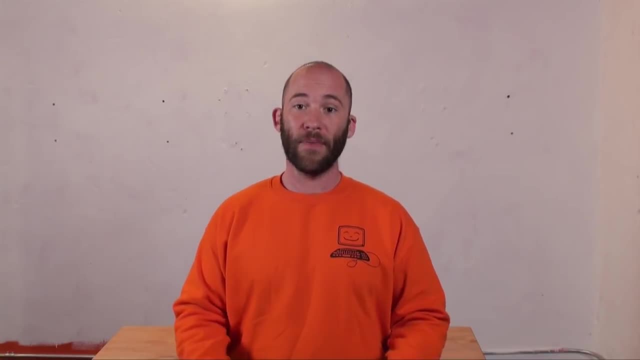 that you get. So when you get a Windows 2008 server, not only do you get the server operating system, but the file server is already built in The web server. so if you wanted to have a website- IIS- it's called Internet Information. 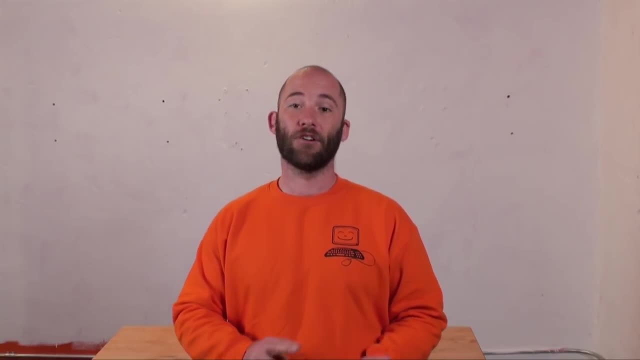 Server is already built in. FTP server is already built in. Terminal services server is already built in. Active Directory server is already built in. So if you get a Windows 2008 server, most of the server functionality that you will ever use is already built in to that server. 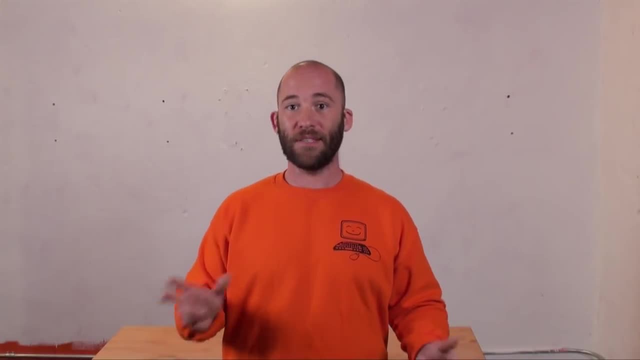 If you are using Linux, you have to install all of these different pieces of server software individually. So when you create your Ubuntu server, when you start it up for the first time, it's not going to do a lot. You have to install and set up the FTP server. 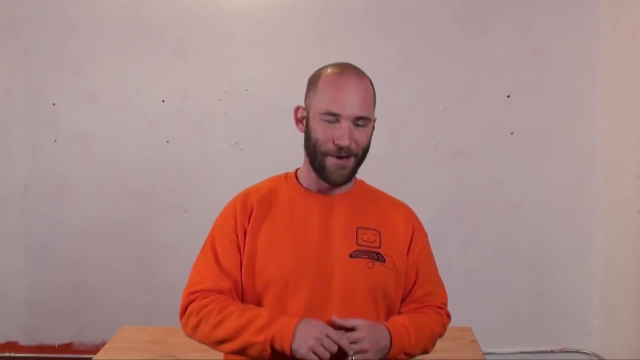 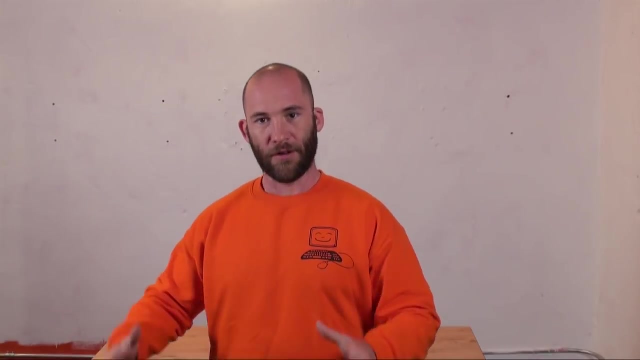 You have to set up the Apache web server, You have to set up the database server. That stuff is not already included in the software. And again, if you don't need a server, a server, you know a server that's going to deal with. 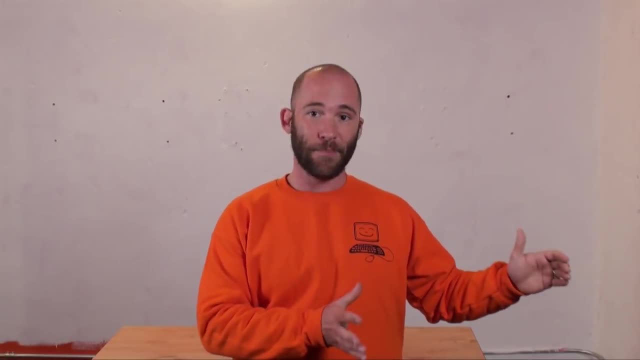 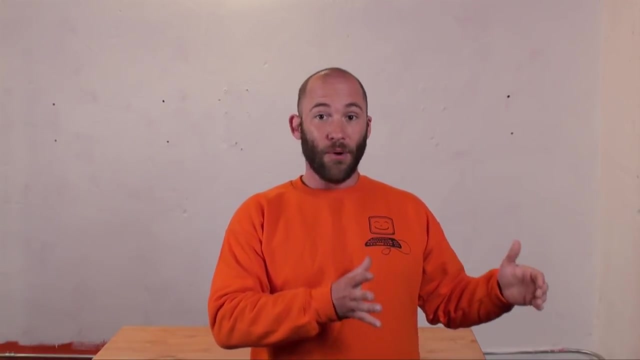 a thousand or ten thousand people. you're just going to use a little Windows XP computer. there is software that you can buy to install on that little Windows XP computer so that it can have a lot of the server functionality. So if you want a web, a fully functional web server, on a Windows XP home computer, you 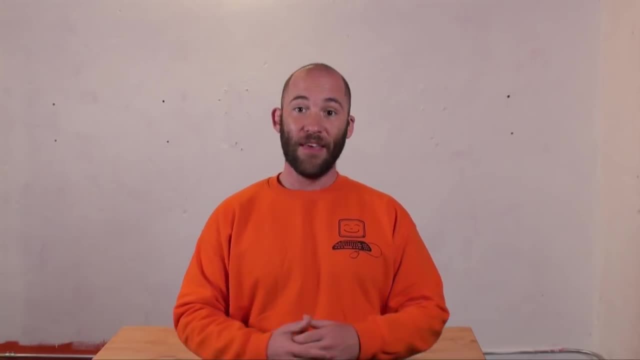 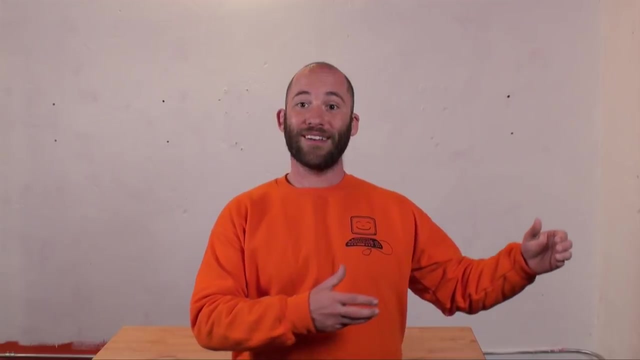 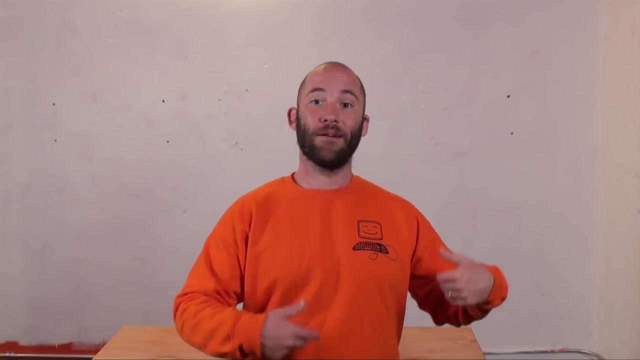 can download for free something called Apache web server And this makes that little Windows XP desktop computer a full web server where you can run a real website off of it. Or you can install MySQL database so it can be a database server. You can install something called FileZilla server so it becomes a full fledged FTP file. 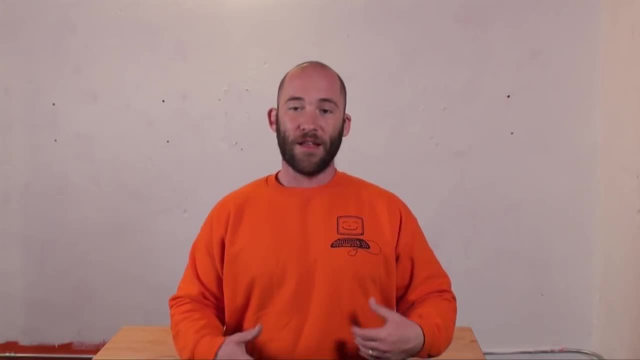 server. So what I want you to realize as we go into all these different things that servers can do, is that all these functions can be on one box, so you can have one physical server that does all of these things. If you buy a Windows 2008 server operating system, most of this functionality is already. 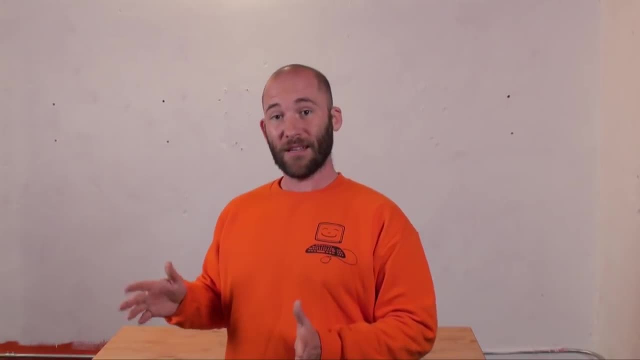 built into it. basically, you just have to turn it on. If you're using Linux, you're probably going to have to install all of the functionality that you want it to do, And if you're using one of the desktop operating systems- Windows XP, Windows 7,, Windows Vista- 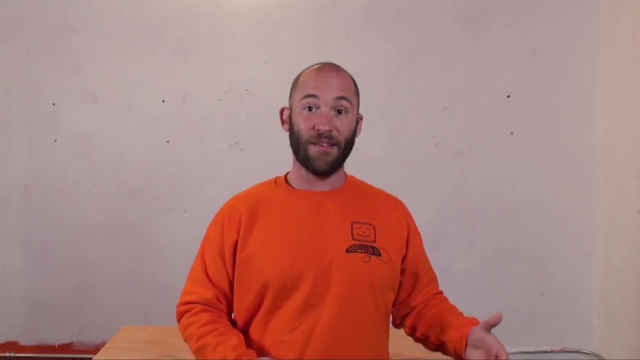 a lot of the functionality. you can get a lot of the functionality by installing additional pieces of software onto it, Like I say, FileZilla FTP server, If you wanted to use it as an FTP server, Or Apache to turn a Windows Vista computer into a full fledged web server. 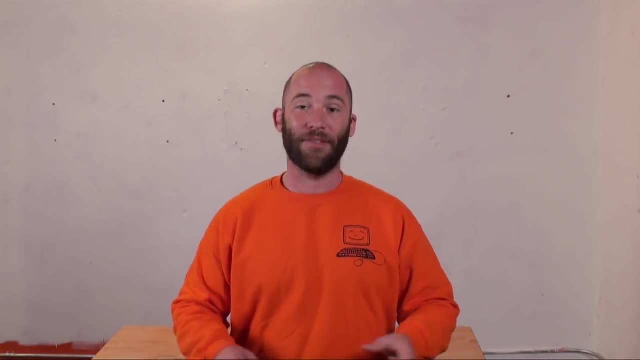 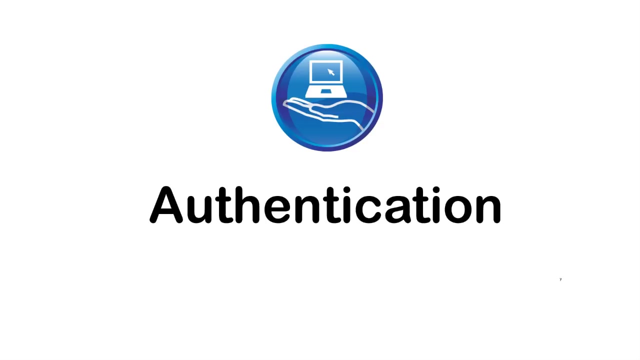 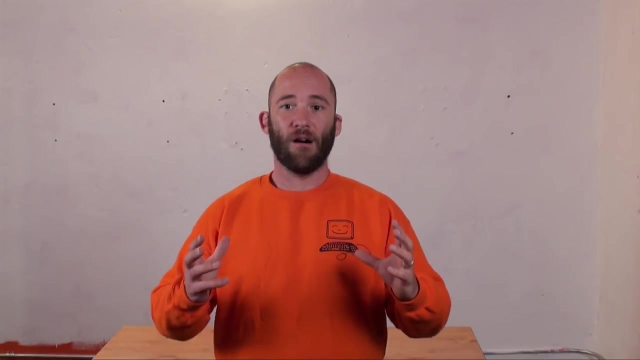 So all of the things we're going to talk about is basically software. Think of it as like Word and Excel and PowerPoint, but the server variety. So with that, let's go in and talk about the different things that servers can do. Now, one of the functions that most people are most familiar with are the security functions. 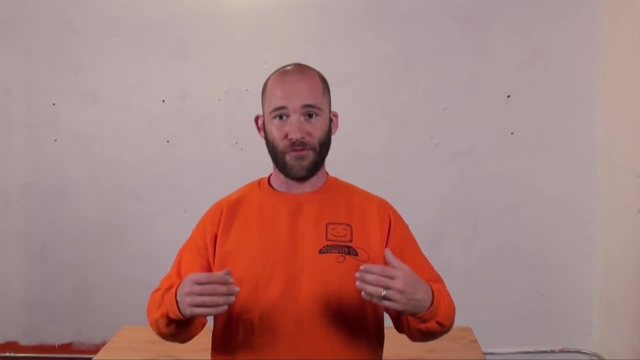 that a server can provide for your network. If you've ever gone to a university, if you've ever worked in a major corporation. when you sit down at your computer, you have to log into the computer. And not only do you log into the computer, but you actually log into the network. 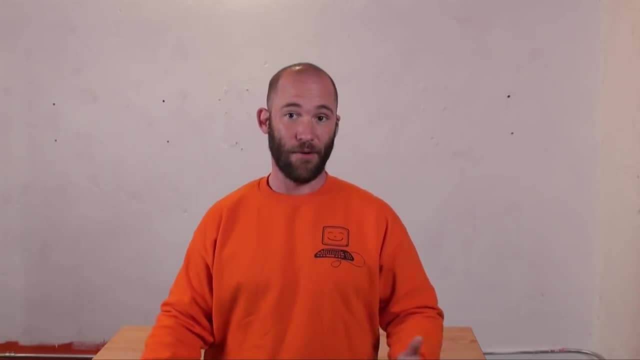 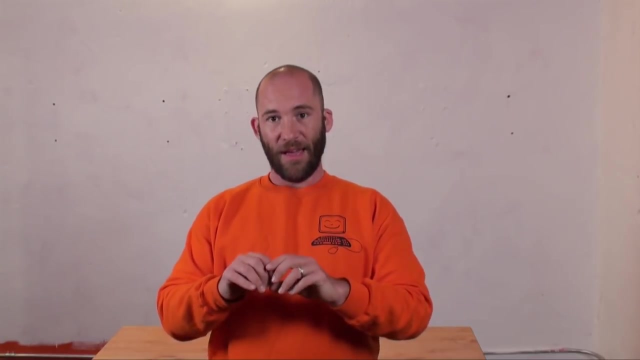 So there is a server on the network that allows you access to the network And this is something called an authentication server. Now in the Windows world they use something called Active Directory. so you have an Active Directory server Basically, when you sit down to log in to the network- your username, your password. 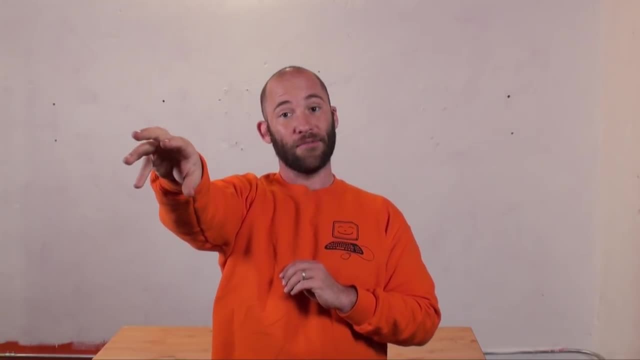 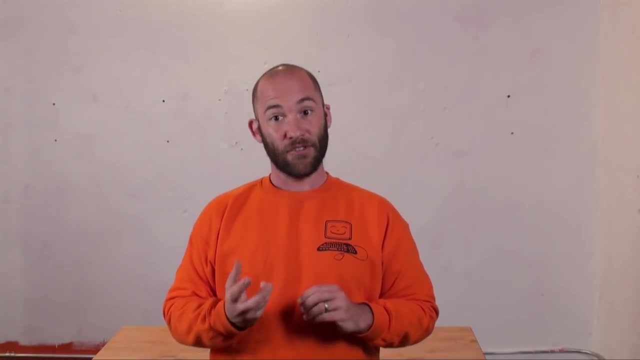 goes up to that Active Directory server. That Active Directory server makes sure everything is okay And then it gives you something called an access control key digitally. This access control key says what permissions you have to do things on the network. So basically you log in. 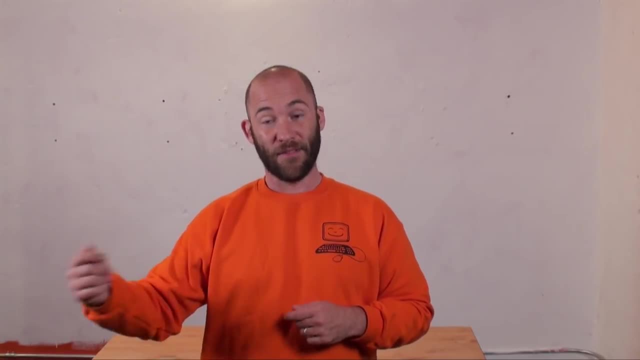 It gives you this key and then you can then get into the files and folders that you're supposed to gain access to. and you're not allowed to get into the files and folders, You're not allowed access to them. So in Windows this is called Active Directory and this is provided by something called domain. 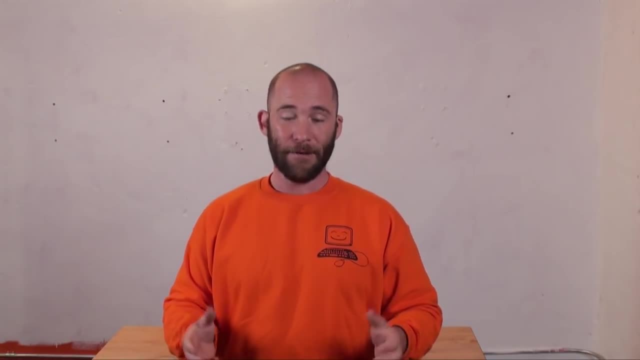 controllers. Back in the day, back with Windows NT, there used to be something called primary domain controllers and backup domain controllers. Nowadays there are just domain controllers. There's something called replication. We'll talk about it in a different class. You go to any one of these domain controller servers. 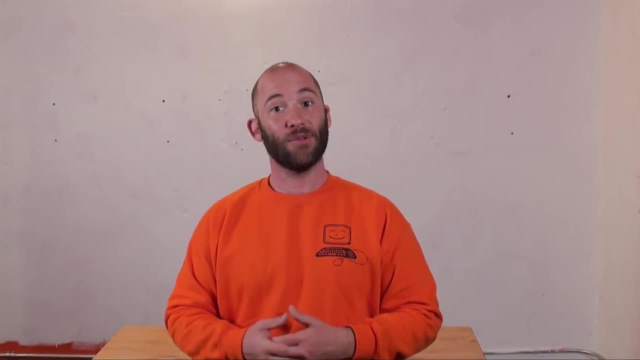 You give it the username and password and then it gives you an access control key to allow you to get to whatever resources you're allowed to use on the network. If you're using Linux, they have something called a Samba server S-A-M-B-A. 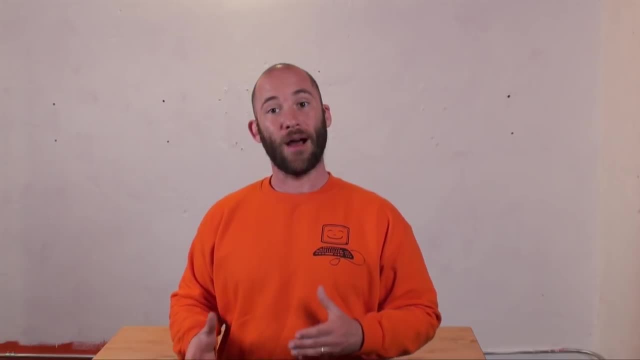 It works much like the old Windows NT primary domain controllers, so it's not as robust and it's not as fully functional. It's not as functional as the new Windows 2008 Active Directory servers, but it does allow you to have one single place where people can log into on the network and get access. 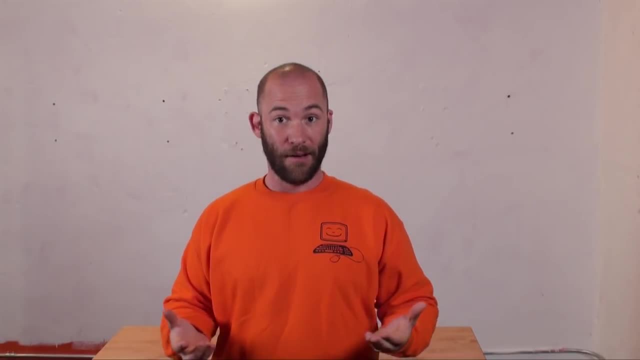 to different resources. Active Directory was created by Novell originally, and Novell Network also has an option for this type of server. So the first type of server that you're probably used to dealing with is the security, the authentication, server. Okay, 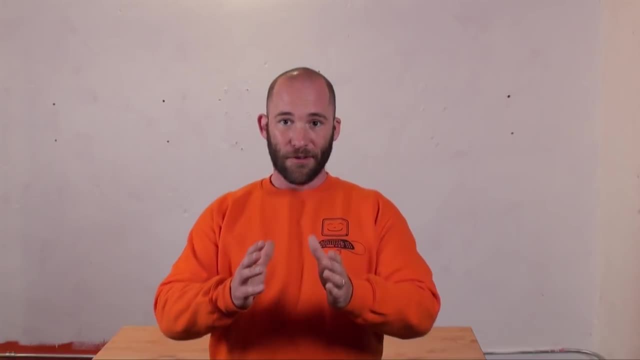 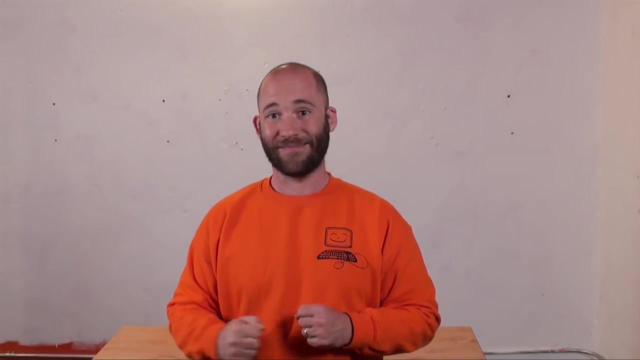 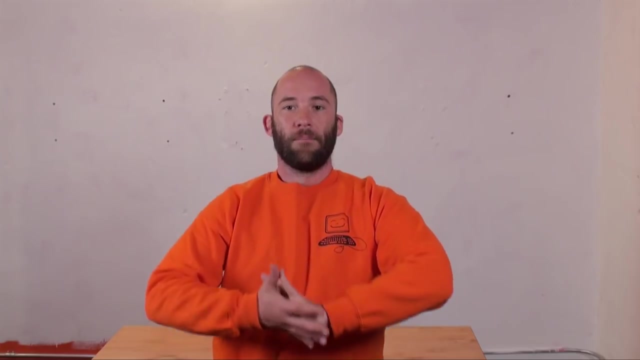 So this allows you to send your credentials, your username and password, go to it and then it sends a key back to your computer to allow you to get to accesses and resources on the network. That's all it does. So we've talked about the authentication. 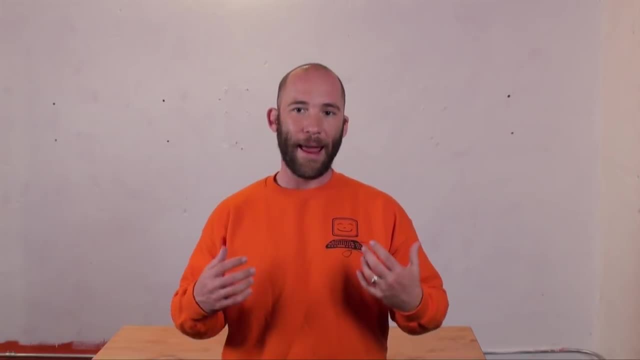 The next type of server that you're probably most familiar with is something called a print server. So back in the day, back 15 years ago, What you used to do is you used to have a computer on the network. You would plug a printer into that computer and then you would share the printer to the 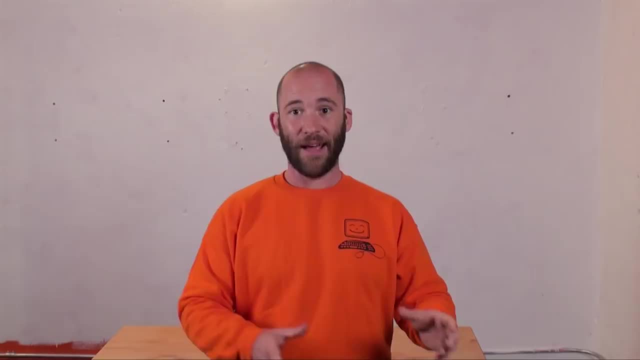 rest of the network. So you could have one printer connected to a computer and then a hundred people could then, through that computer, print out. So that was a print server. Like I said back in the day, they had very, very specialized servers. that all that's. 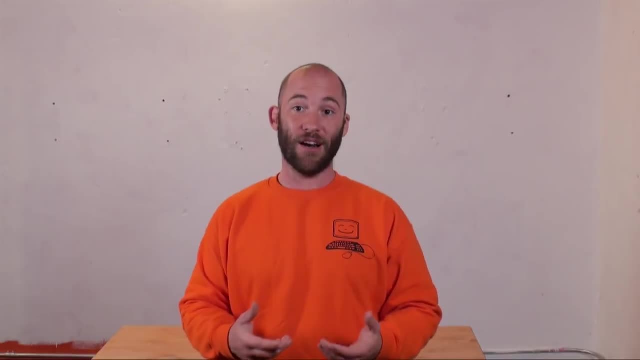 all they did. So all a print server does is allows you to share a printer. That's all they did. So you could share a local printer on the network. Well, that was kind of expensive, So the most common solution after that was HP came up with these what were called jet. 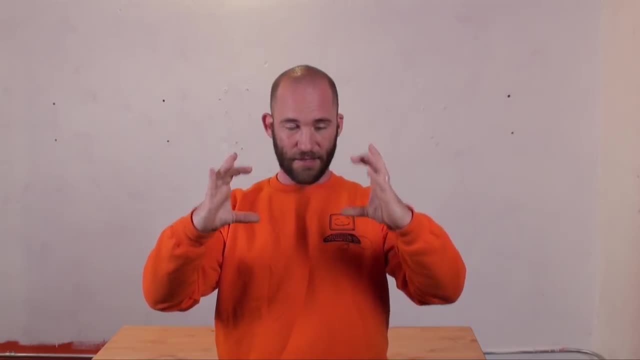 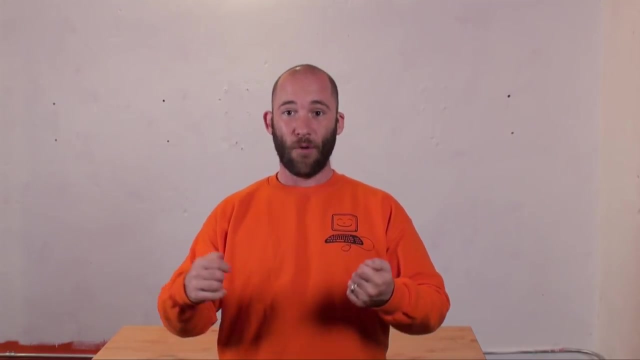 direct print servers. So there were these little gray boxes of they kind of look like little switches that you might buy at Best Buy right now And what you could do is it had one port for the network and one port for an HP printer. 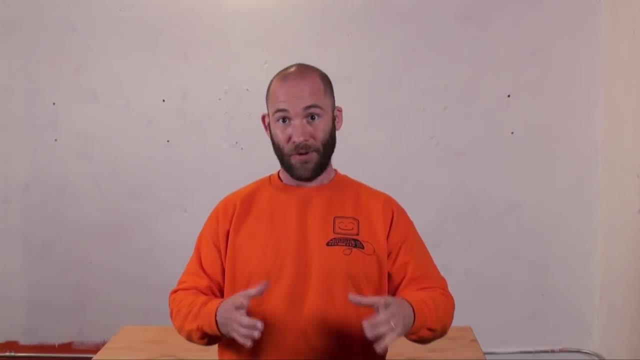 So this HP jet direct printer, So this HP jet direct print server, would act like a normal print server and allow people to print to that printer, So you could have a hundred people basically sharing one printer. As time went by, that print server, that HP jet direct print server, became an HP jet. 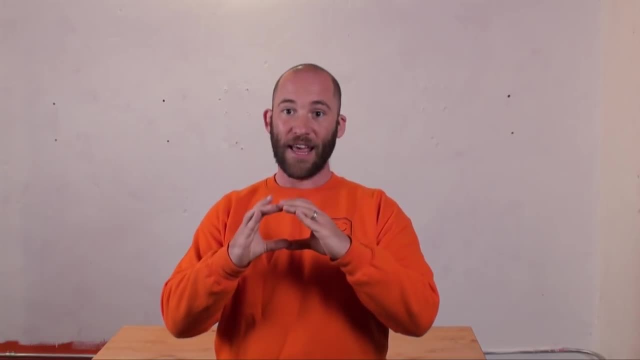 direct card. So it went from being a box to just being a card that you could slide in as an additional accessory to the newer HP printers that came out As time progressed. beyond that, Then the print server got built in to the printer. So now printers have built in print servers. 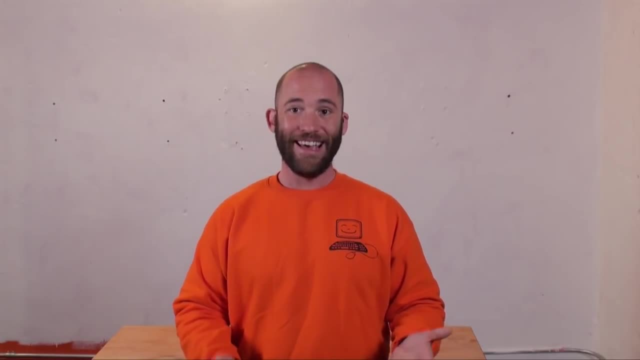 So just keep this in mind: when people are talking about print servers is now in 2010,. most of the time, print servers- the actual print server- is built in to the printer and you just plug the network cable directly into that printer. It works on the same ideas as when you used to have a computer plugged into the printer. 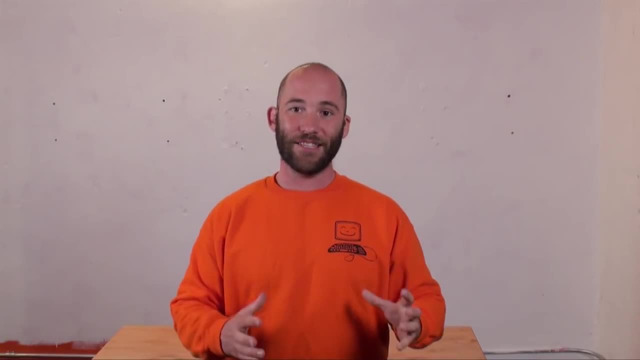 The printer is just all now into a single printer. So that's what a print server is, is. it's simply a computer that allows other people to print through it. Nowadays you may still like if you have a small office, or in your home you may have. 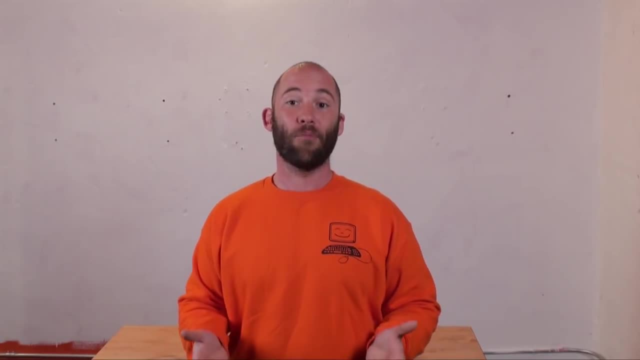 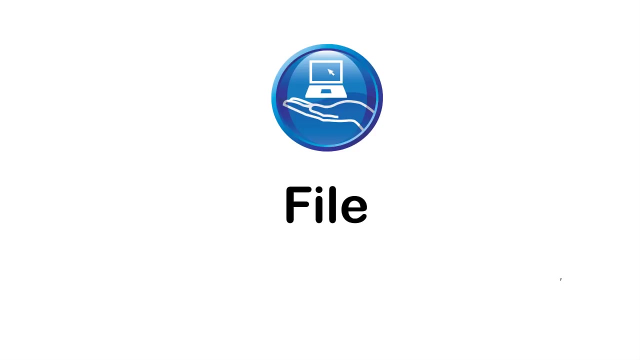 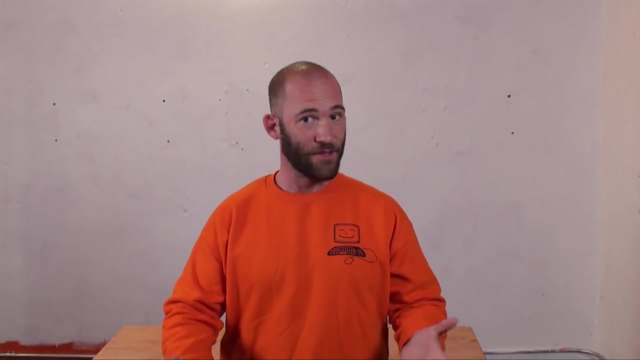 a desktop computer that acts as a print server. So you may have a print server that way, But that's all a print server is. So pass the authentication server and the print server. We then have the file server, which you're probably very, very used to. 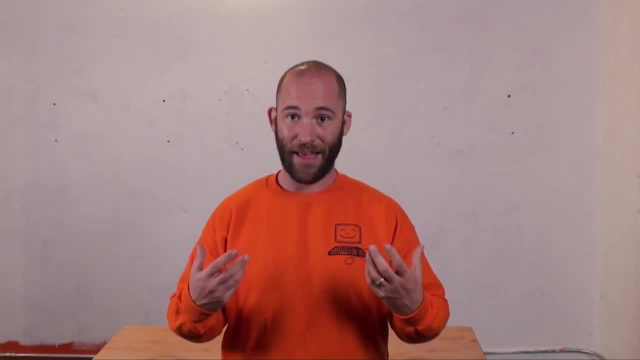 This is where you have a network share. So you have a folder that's shared on the network and everybody in the office can just get into that share and open up or modify, do whatever they want to the files that are inside the share. That's all a file server is. 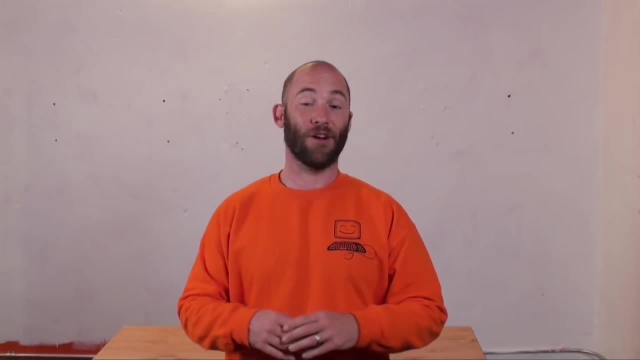 It is simply a computer that has a share folder or shared folders with shared files That people on the network can access. Yeah, there's just not a lot to it. That's all there is. So now we start coming to things that you may not think about, that you may not be used. 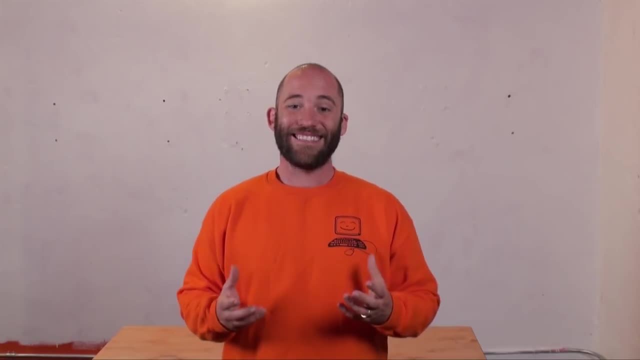 to thinking about with servers. The next thing is web and FTP servers. So this is a server that you go to and it presents you a website. So this is a server like everymanio com. When you come to our server, it gives you a website. 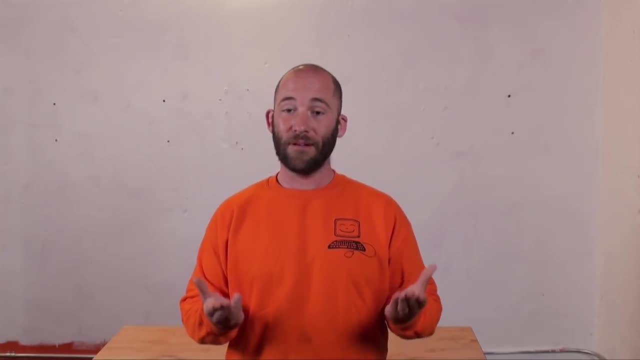 There are two main pieces of software available that are for websites. There's either Apache A-P-A-C-H-E, which is open source and free. It can be used on any operating system to allow that operating system to be a full fledged. 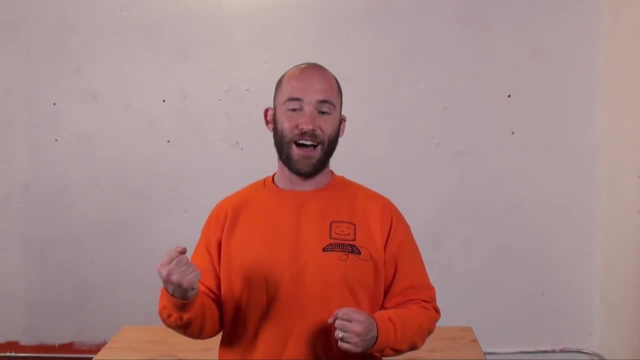 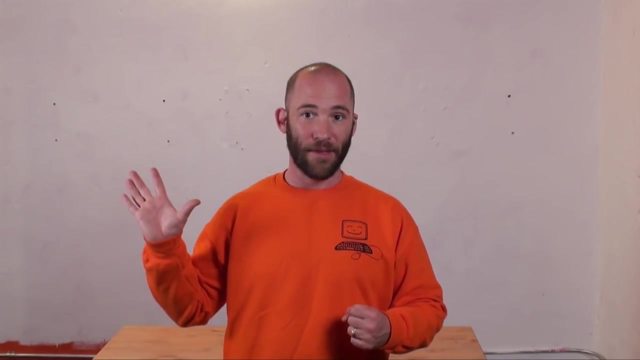 web server, Or in the Windows world, there is something called IIS Internet Information Server. There is a version built into all Windows operating systems If you deal with Windows Server, so Windows Server 2008 operating systems, you have the. 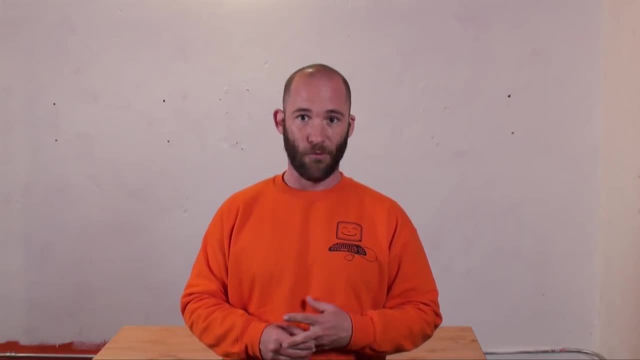 full fledged version of IIS and you can present a world class website using that. If you have Windows 7 or Windows Vista or Windows XP, they have a version of IIS built into those too, but it's not as robust. They don't allow you as many connections. 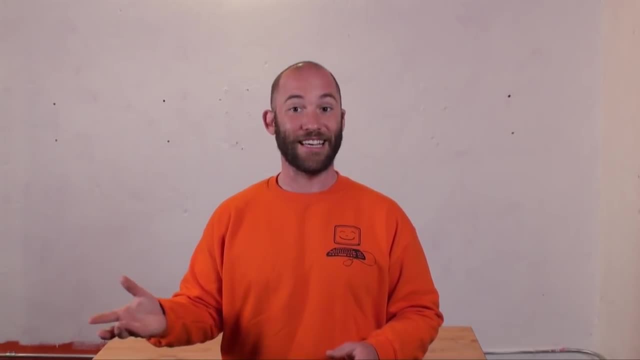 Don't quote me on it, But I think they only allow like 25.. 20 concurrent connections at a time, So only 20 people can be on your website at any one time. So the two types of web servers out there are Apache and IIS. 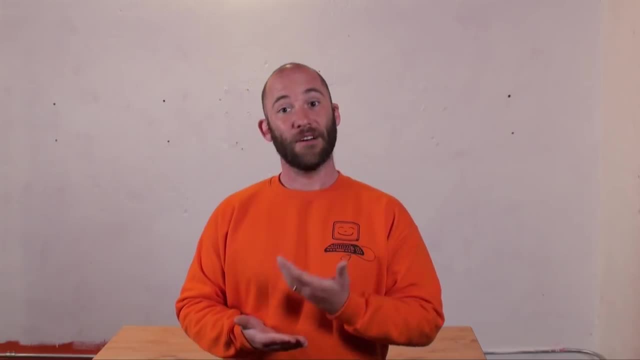 Again, Apache can be installed on Windows. it can be installed on Macs. it can be installed on Linux, it can be installed on anything. IIS can only be installed on Windows computers. Now, along with the web server that provides you websites, you also normally have something. 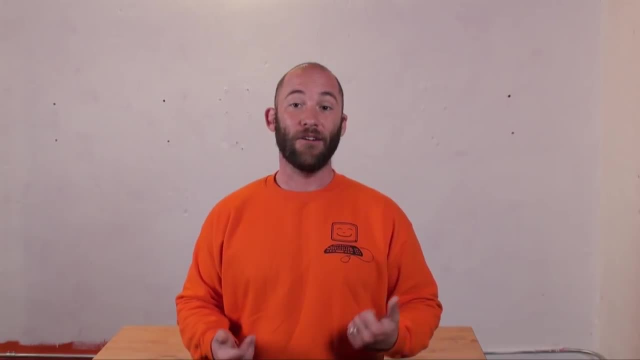 called an FTP server. This is something called Firehose. Okay, File Transfer Protocol. File Transfer Protocol allows you to transfer files from one place to the other, So if you're trying to upload files onto your website, you would use FTP. 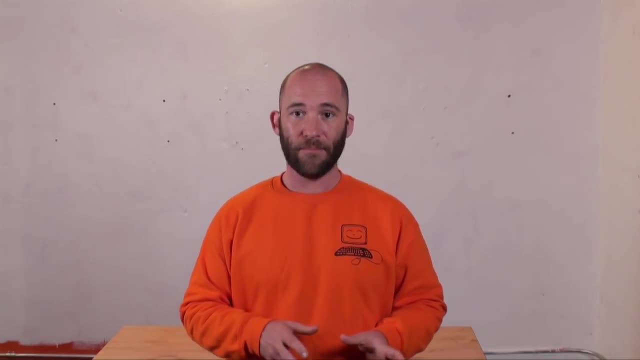 This is different than a normal. like a file server, A file server uses a special protocol in order to transfer files back and forth. FTP uses a different protocol to transfer files back and forth, But normally Um FTP servers are servers that normally sit on the internet and allow you to upload large 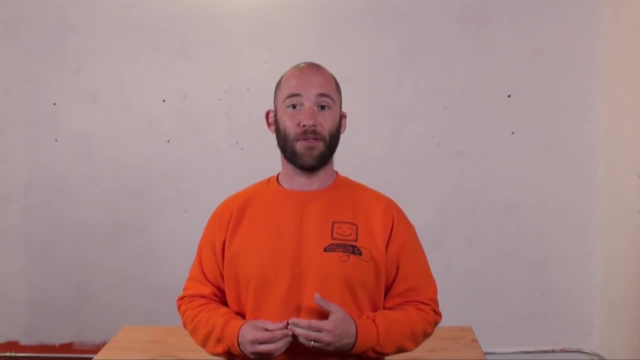 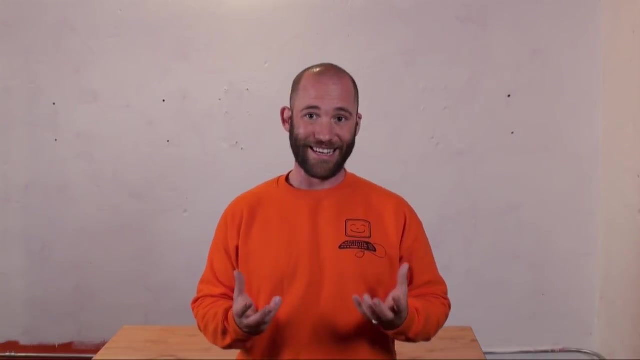 files to them for whatever reason, And they're normally included with web servers. So after web servers and FTP servers, we now have mail servers. So these are servers specially designed or software specially designed to route email. So what you do with an email server is you set it up in your office. 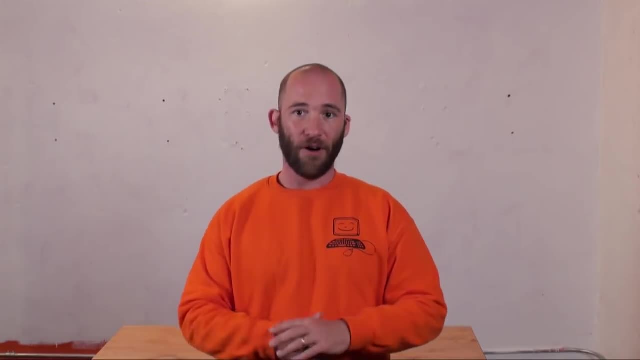 And then all the email for your company. so if you have 100 people, all the email for your company will go into that one single server and then that server will decide what to do with it. It'll send it out to wherever it needs to go. 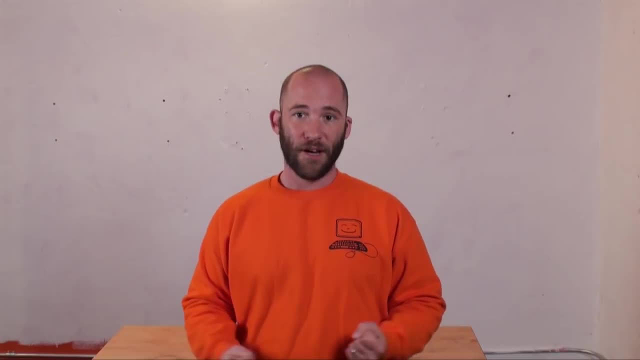 Most people are used to Microsoft Exchange servers. So with Microsoft Exchange servers all the email comes into the Exchange server And then whenever anybody logs in using Outlook, they're able to get all of their email off of that server. Or, if they have smart phones or, you know, iCloud. 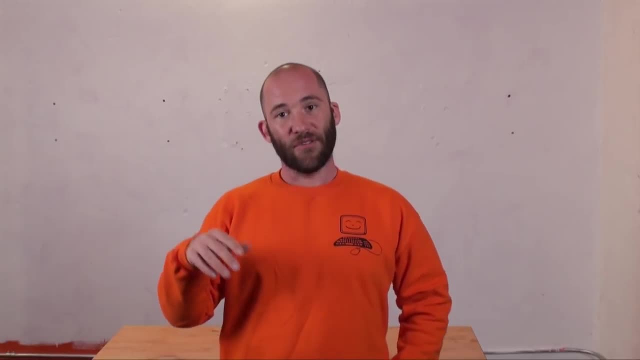 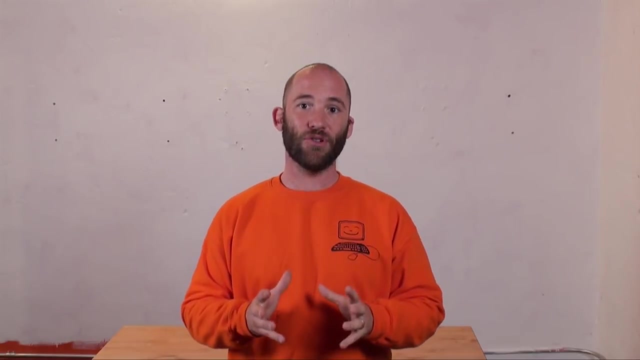 They're able to get all of their email off of that server. Or if they have iPhones or such, That Exchange server can also send emails to whoever it needs to go to, to their smart phones. So the email server actually routes email for a company or for an organization. 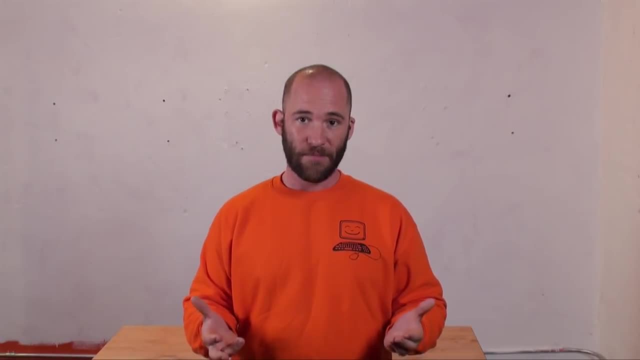 The most common email server again is Microsoft Exchange. In order to use Microsoft Exchange, you have to have a Windows server. It will only run on Windows. If you don't want to use Microsoft Exchange, there's a whole slew. There's a whole slew of other types of email software out there. 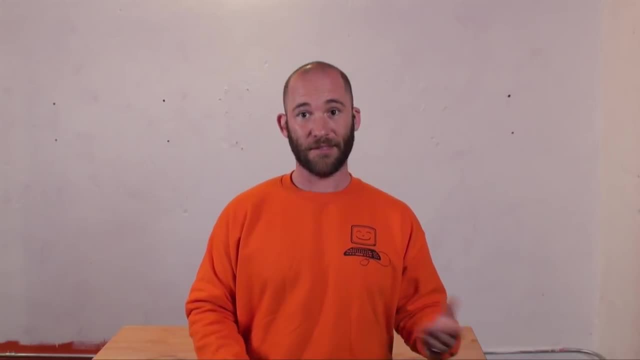 Some of it's free, Some of it's very expensive, Some of it only runs on Linux, Some of it only runs on Windows. It all depends on what you decide to use and what you decide to buy. But the main thing is what mail servers do. is they take all the email for an organization? 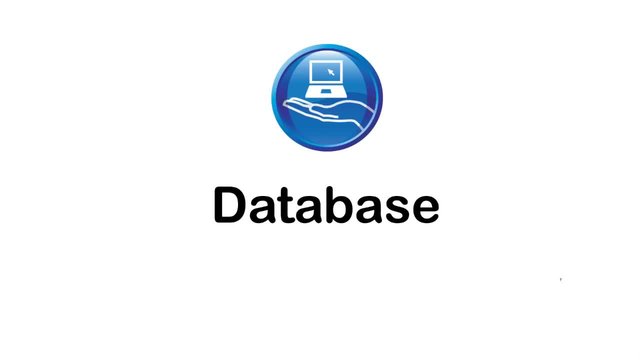 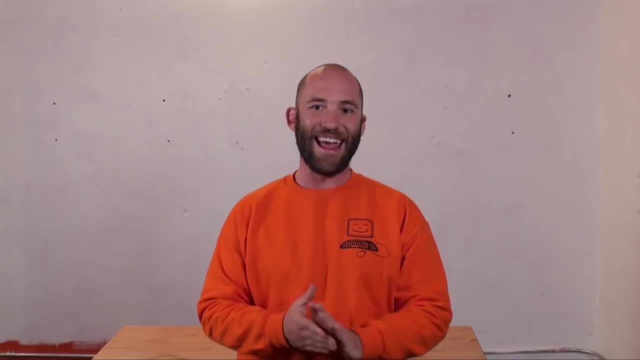 and then they route it to the right people. So the next type of server is email. Next type of server is a database server. So databases, all they do is store data. They store data and allow outside applications to put data into it, to pull data out, to. 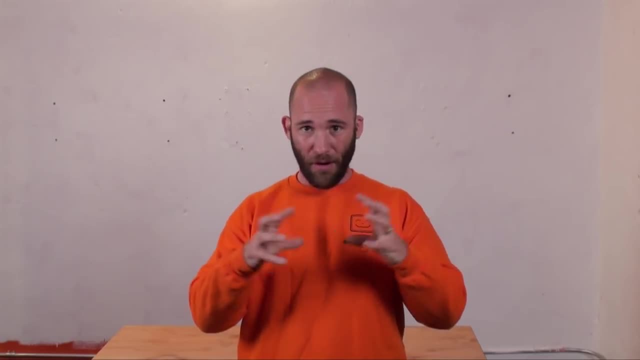 manipulate the data. that's there, But all databases do. all they're worried about is data. They don't have fancy interfaces, They don't look cool, They're just basically, you know, they're like a lot of things. All you get is a little DOS prompt. 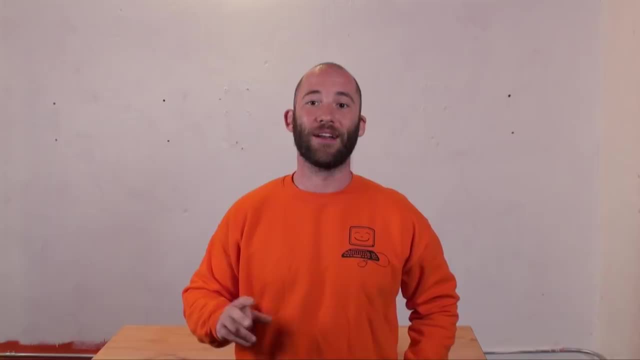 And you have to. you know you have to do a lot of things, You have to type in these long SQL statements if you want to get anything out of it normally. But outside pieces of software can't interact with a database server And, like I say, they can either put in data or pull out data. So if you have a customer contact database, you would use this. Let's say, if you have a ticketing system, ticketing systems use databases, So it gathers all the information from a ticket and puts it into a single database. Most of the time, database servers reside in the same server. 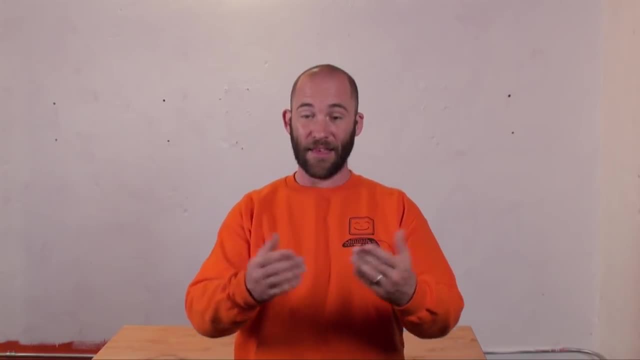 As a web server. So let's say, like this website, Everyman IT has a database as part of the website. So there is a MySQL server installed alongside the Apache server software that runs the website. But all databases do. is they just database servers do? is they just handle data? 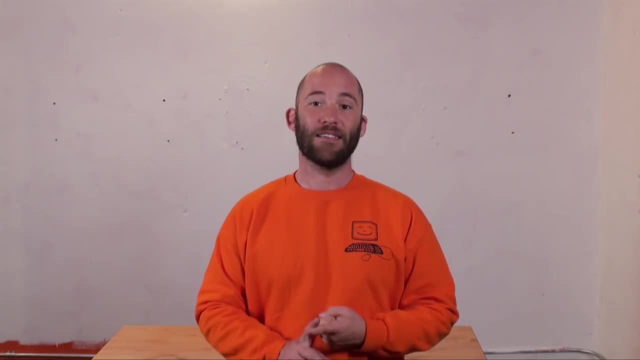 The most popular database software in the web world is something called MySQL, which is free and open source, And it's called MySQL. There is also Microsoft SQL, which is not free. It's very expensive. It will only run on Microsoft SQL servers. 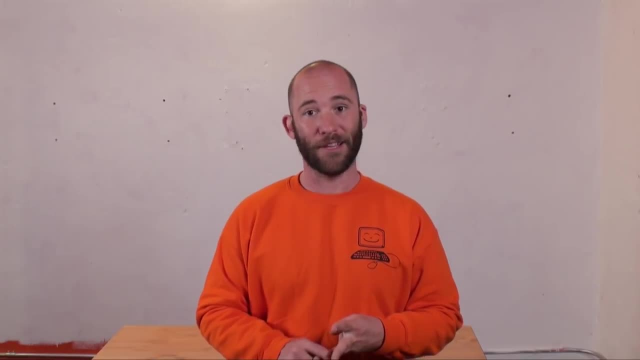 And then of course you probably also know of Oracle, which again is horribly expensive and runs on all of its own stuff, But basically all database servers do, is they just they just deal with data, They just, they don't. they don't really do anything fancy with it. 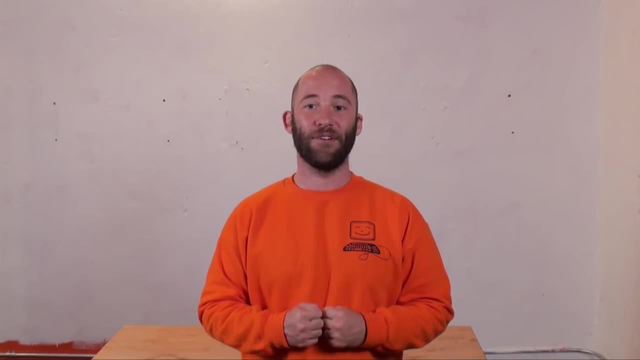 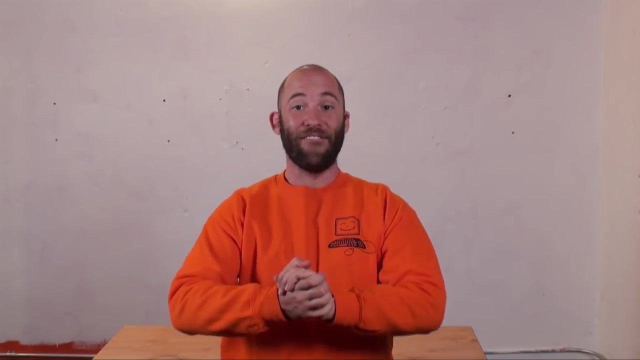 They just store it and allow you to access it or put stuff into it. So the final type of server that we're going to talk about is a remote access server. So nowadays these are normally VPN servers or virtual private networks. Back in the day they used to have dial-up servers that would actually have little modem. 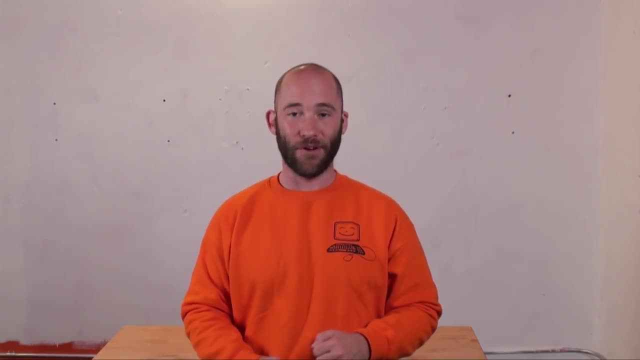 cards in them and you could actually dial into the server. But nowadays we're normally just dealing with VPN. So what the remote access server does is allows you. It allows you to connect to the server and then, from there, get access to the rest of. 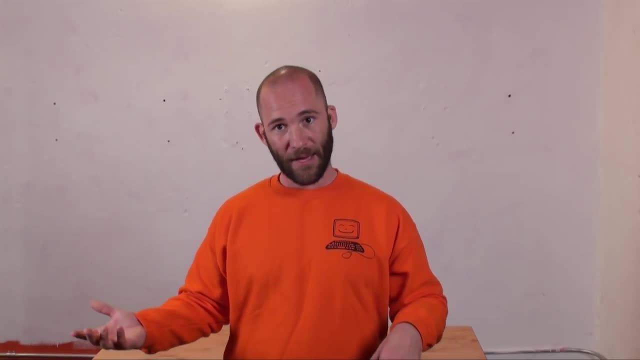 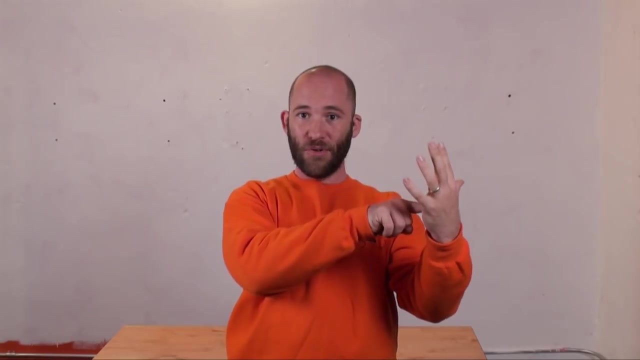 the network. So if you're out on the internet and you have a piece of VPN software and you have this remote access server- so it's a VPN server- you can connect through the internet to that server and then, once you've connected to that server, you get the resources that are that. 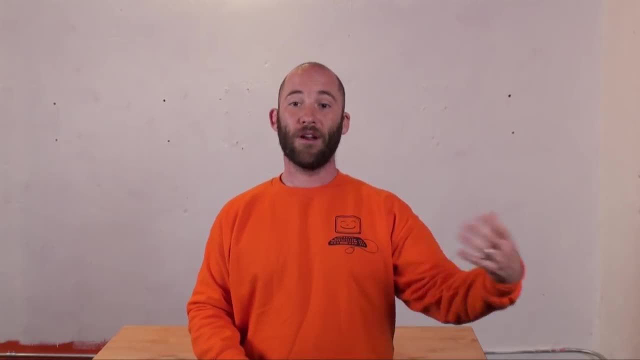 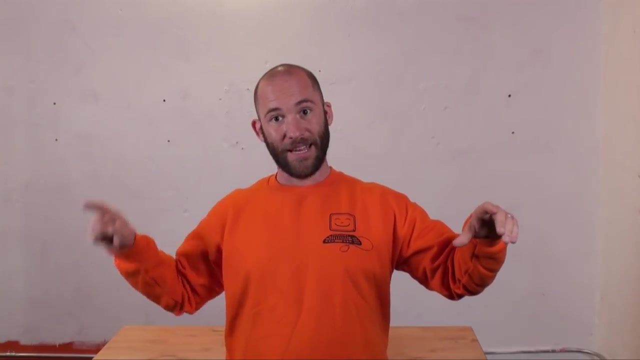 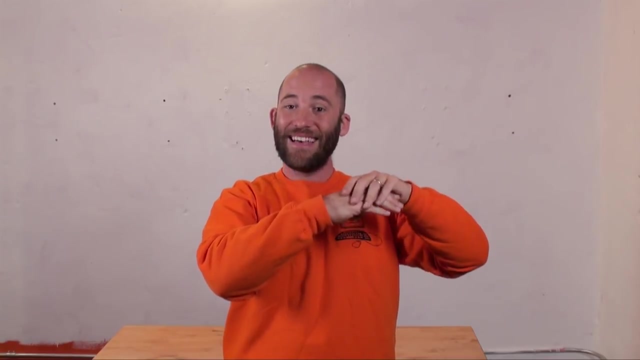 are in in that, that local network. So imagine if you wanted to print to a printer that's that's in an office 500 miles away You would use, you would connect to the server in that office using something called VPN and then, once you've connected to that server, it's as if you're on that local network and 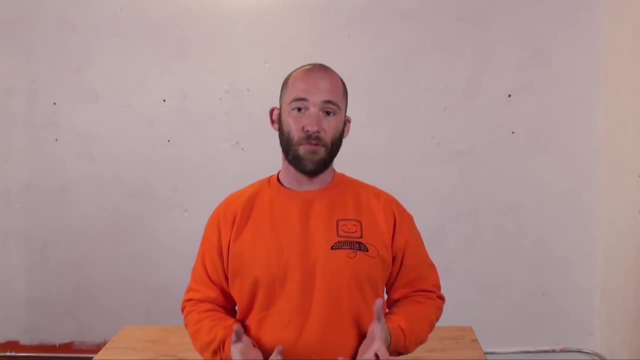 so you could then print to that printer. But basically all the remote access servers do is they allow you to connect to the internal network from the outside world, from the internet, And then, once you've done that, then it's like you're. you're basically as far as the network. 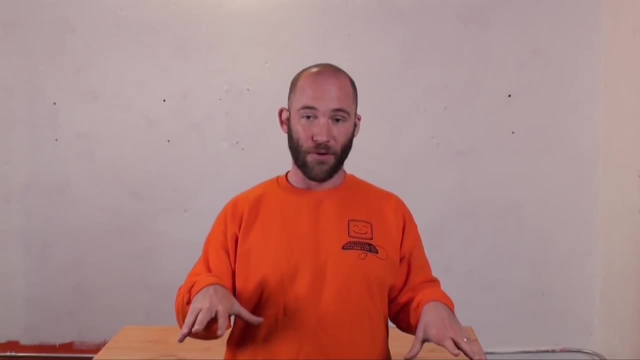 is concerned, You're local. you're, you can use all the local resources. you can print to a local printer. you can get your email just like you're in the building. That's all a remote access server is. So we've discussed a lot of things in this introduction to servers class. It may take a while for it to all, to all digest so so. so don't worry. Servers are a whole new world compared to simply dealing with with desktop computers. All servers are, remember, all. all a server is just a normal server. all a server is. 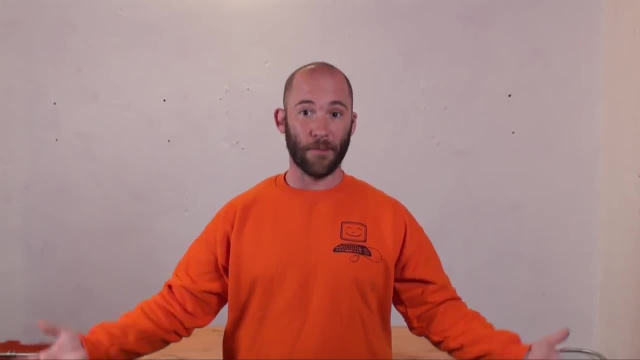 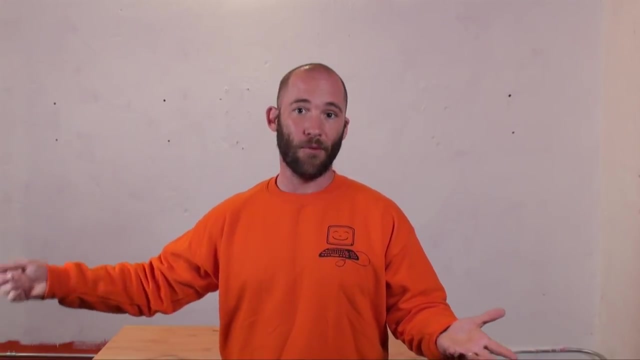 is a computer that provides services to other computers. So if you, if you have a printer plugged into the back of your computer and you have shared that printer out so somebody else on the network can print to it, then you have a print server. 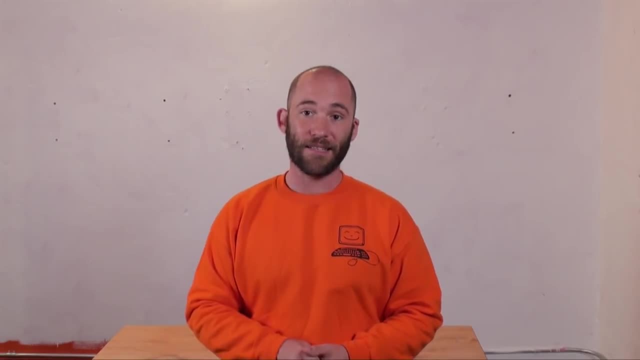 If you have a shared folder on your computer so other people can access that folder, then you have a file server. All though Servers. you know that that is what a server is. it just provides services. There is a difference between servers and servers. 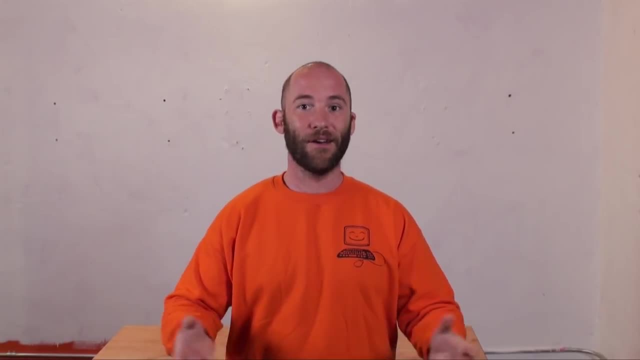 Servers, like I say, you know you can. you can use a Windows XP Home Edition computer to be a basic server. You can have it be a web server. you can have it be a file server. you can have it be a. 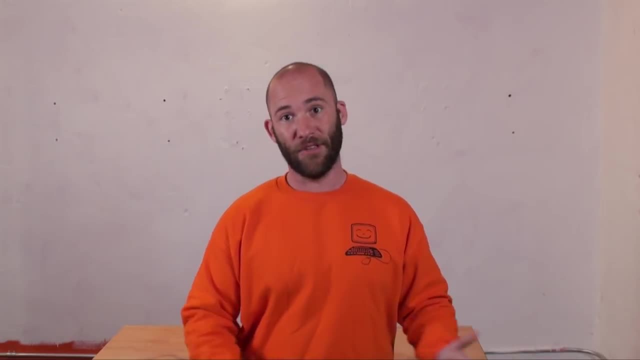 print server. you can have it do most of the functions that that the servers can do, But it's not as stable, it's not as robust and you know there's much more chance that something will go hinky with it. 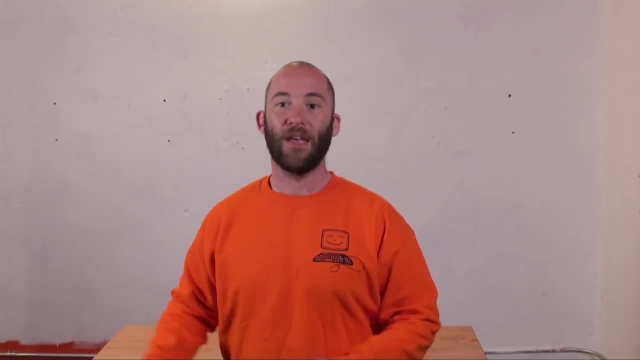 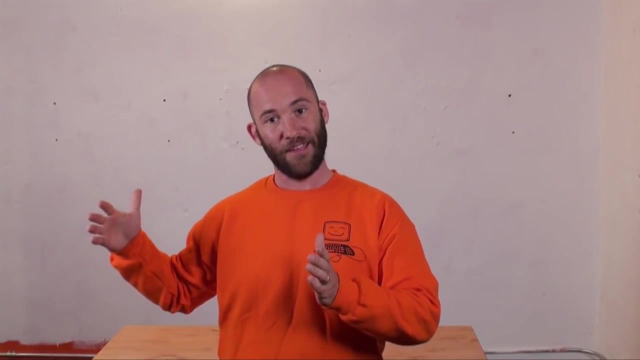 Than with a, with a uh enterprise server. So so you know they're, they're cheaper, but but they're not as robust, Whereas servers, you know, use server operating systems. so, whether it's Windows 2008 Server, 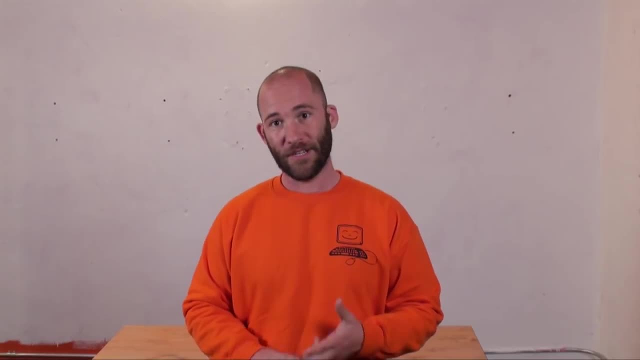 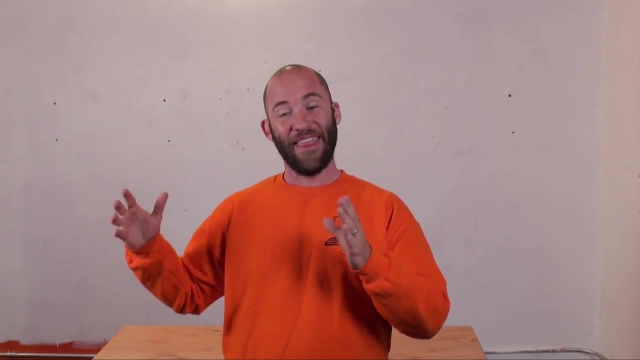 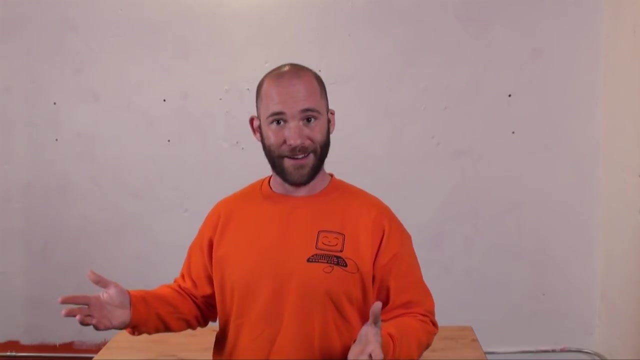 Edition you're using, or whether it's Ubuntu Linux Server Edition or Red Hat Enterprise Linux Server Edition or Mac OS X Server Edition. uh, that server software is built for servers And therefore, of course, uh, if you try to play video games on it, it's not gonna be. 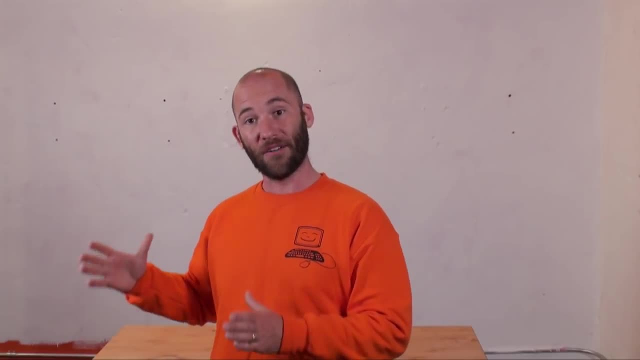 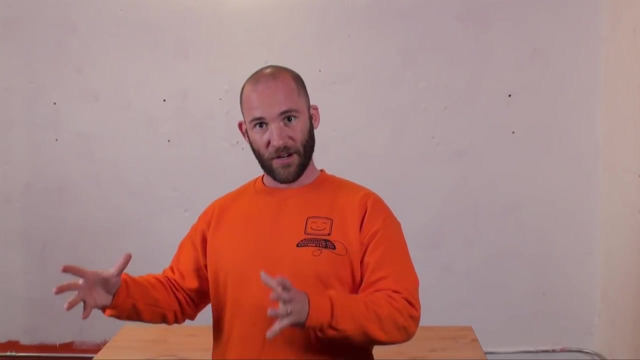 as good as that desktop computer, But it is very good for file sharing, for web, for websites, uh for, for authentication servers and the rest of that. Real servers are meant to deal with, with a lot of of of communication with the outside. 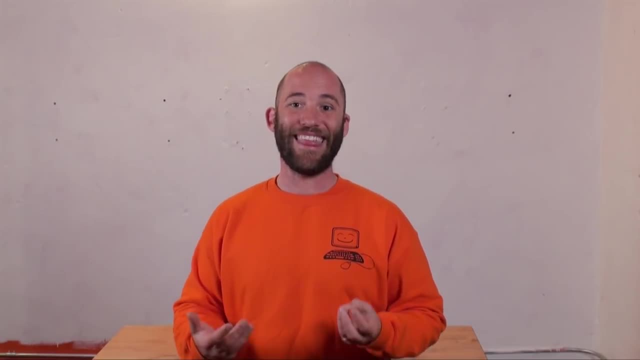 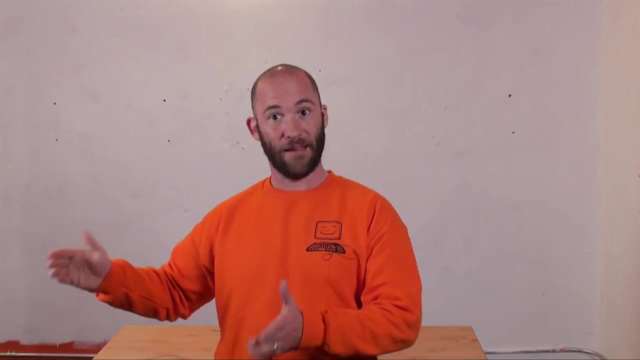 world. Again. an authentication server can deal with up to 10,000, uh clients. So for every 10,000 users you can have, you can have one of these Windows 2008, uh servers. Now there's the- the hardware that we've talked about. 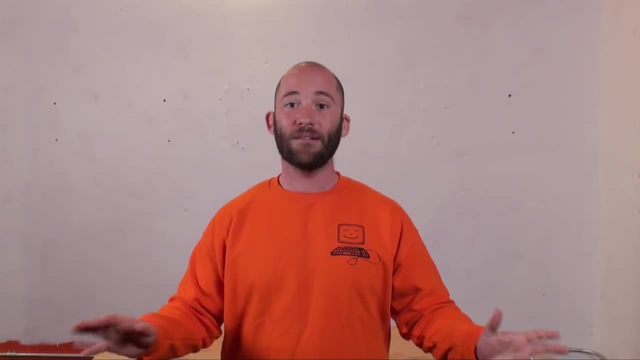 Again, you can use any hardware. You can go out and you can buy a $200 e-machine, or you can go out and you can buy a a netbook and use it as a server if you want to. It doesn't matter. 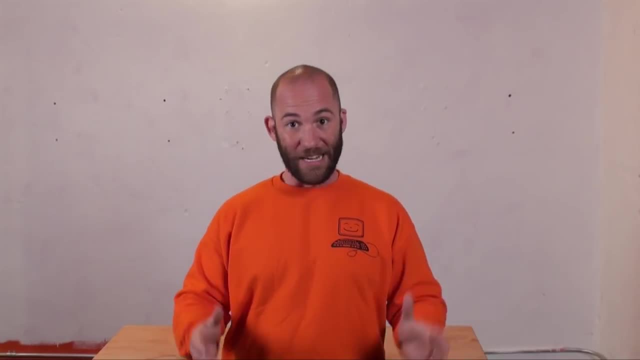 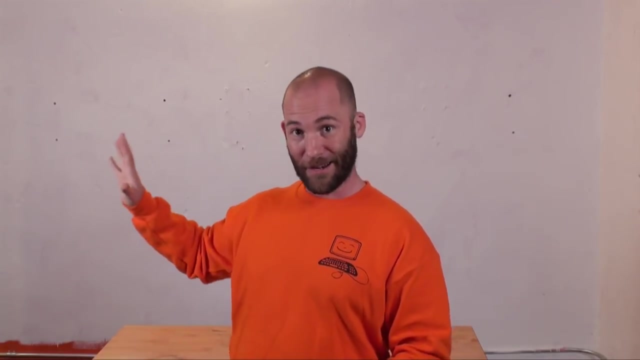 You or well, it doesn't matter. You don't have to use really high quality parts for a server. but if you're like me and you have your server in a data center and and your life kind of depends on it, 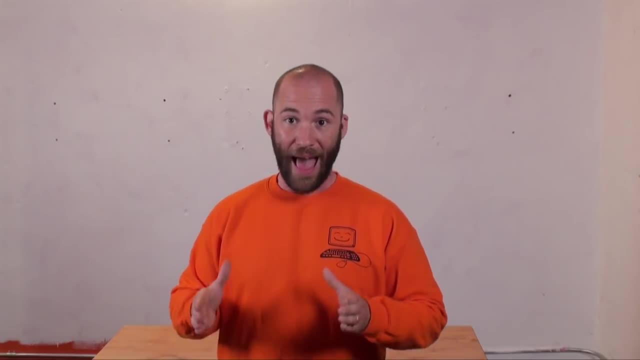 then there there is specificity, Specific hardware that you should have for your server. This includes a Xeon processor, so so a processor designed for servers. This includes redundant power supplies, So if one power supply fails, one of those power module fails, the computer stays up. 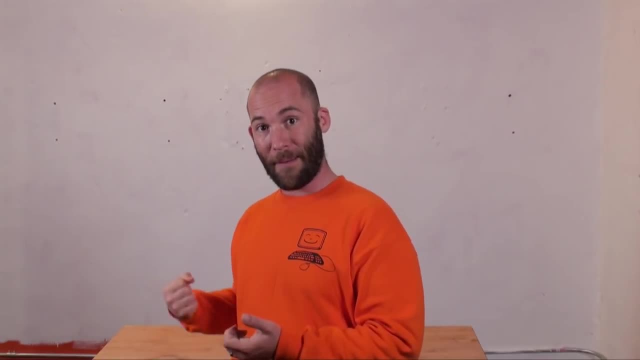 and running and you simply pull out the the bad power supply and put the new one in. This includes RAID. This is where you have multiple hard drives with redundancy, So if one hard drive fails, you can pull the bad hard drive, You can pull the new one out and put a new hard drive in and again the the computer. 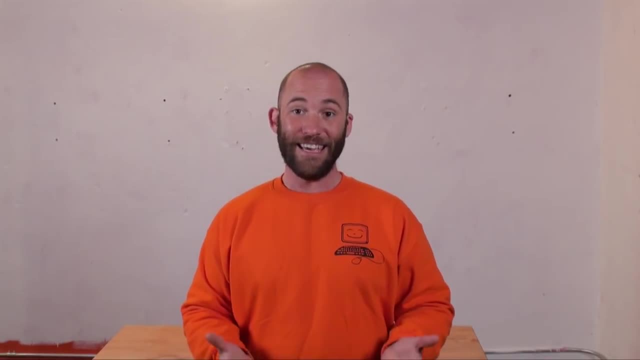 doesn't doesn't go down, There's no problems. And again there's something called ECC RAM. This is error error checking RAM. It actually does tests on itself. Again, this is much better RAM and it ensures you have less problems with your server. 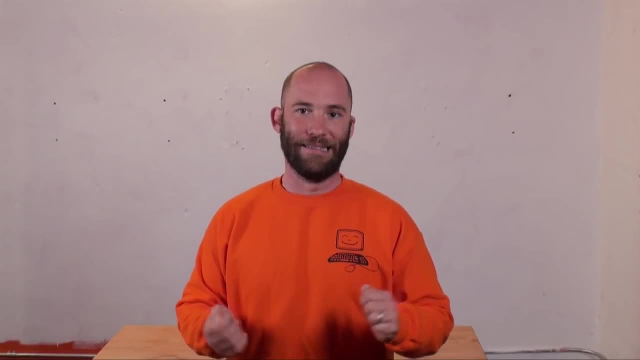 But in my book it is so much more expensive that I'm not going to mess with it. I don't put it in my servers, but it's there. So so the the server hardware, you know, depending on what you're doing, depends on. 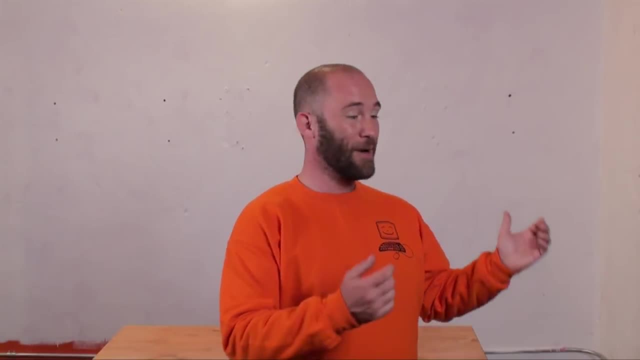 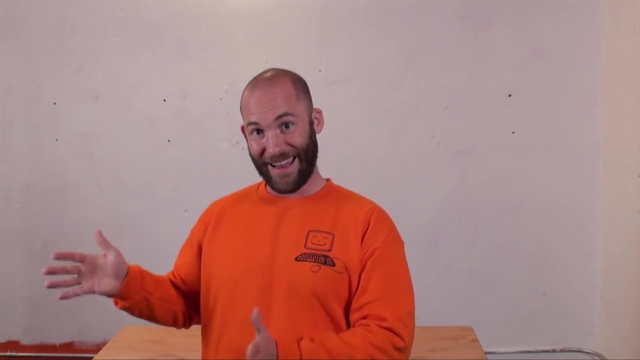 what you want to buy. If you're sharing out some files with five people in the office, by all means buy that e-machine. If you're a, if you have a server that's sitting in a data center somewhere that that can never crash, then then get real server hardware. 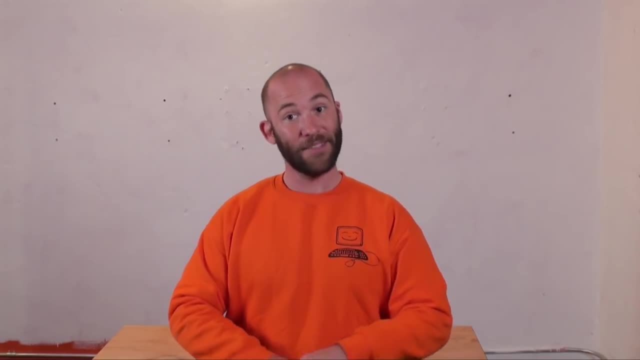 We just talked about all the functionality that a lot of these servers can have. There's even more, There's, there's. there's so many things servers can do, But I gave you the the, the basic rundown of the common things that that most people 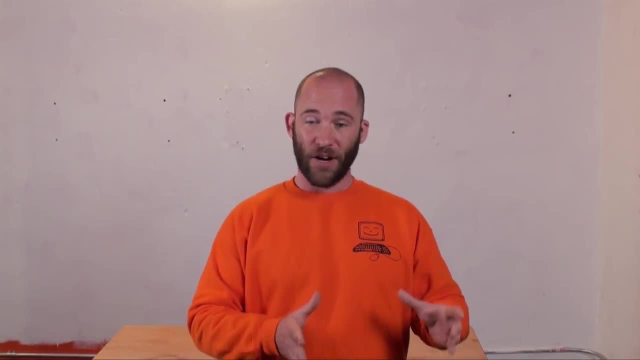 use servers for Again, all these different functions are simply pieces of software just like you would install on a desktop computer. So you know, a desktop computer can do more than Word. It can do Word and Excel and PowerPoint and Photoshop and Firefox. 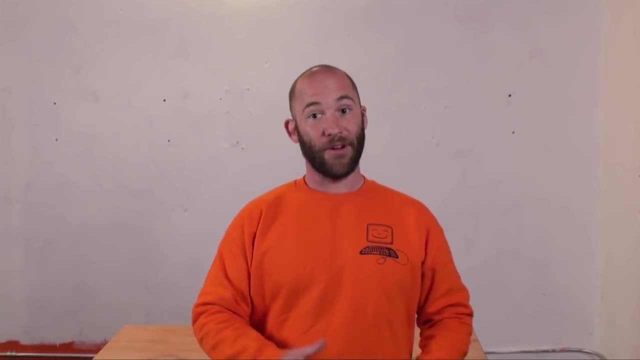 So a server can do authentication and be a file server, and be a web server, and be a database server and be a remote access server, all in one, one box. So don't don't think you have to have one server for each, each of these individual. 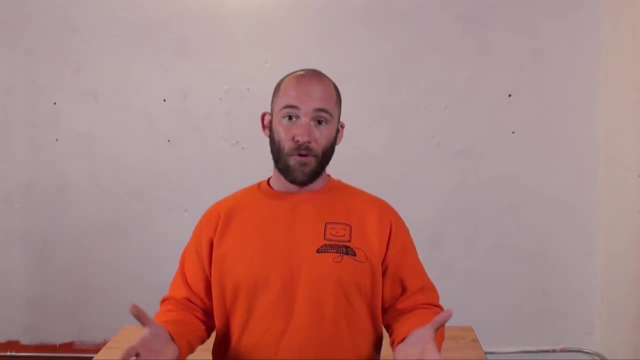 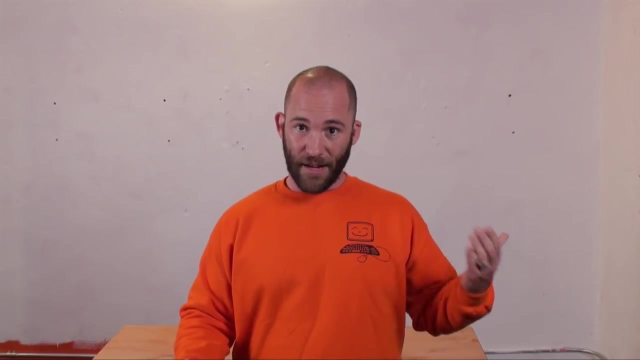 things As we talked about. Those 2008 servers come with all these components already built in and you basically just have to turn them on and configure them. If you use Linux, you almost always have to install these different services separately And, again, a lot of the functionality that I talked about you can install onto a Windows. 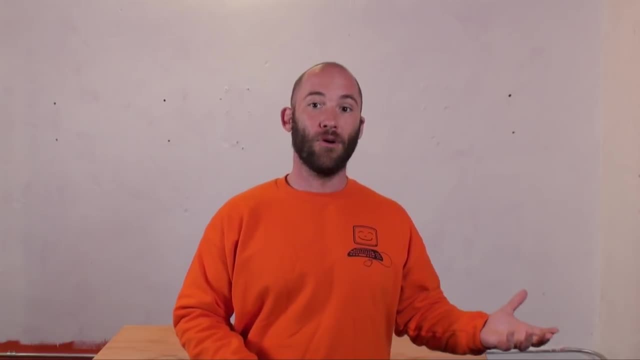 XP home computer, but you do have to download the software to allow that to happen. We talked about the authentication service. All this is is when you log into the network. It's what allows you access to the things you should have access to. 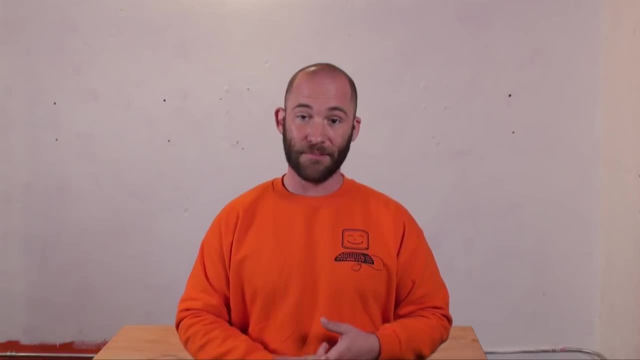 That's all an authentication server does. We talked about the print servers. This allows, you know, one, one printer to be shared by multiple people on the network. We talked about, you know, back in the day, it was a big computer, it was a big actual. 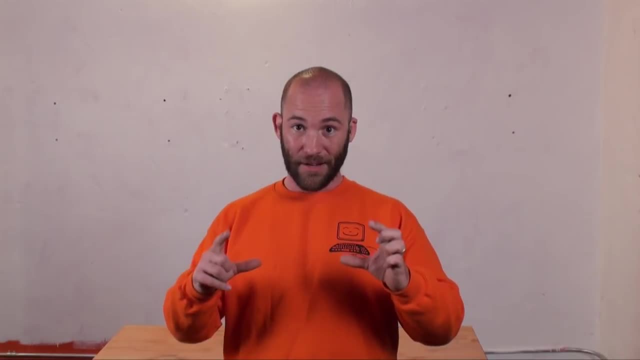 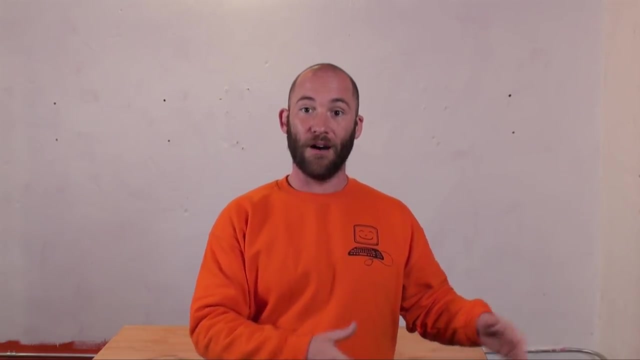 server, and then HP came out with these things called JetDirect devices, and then those became cards, and then that all just got built into the printer itself. So you may see that the printer has an internal print server, And that's what they're talking about. 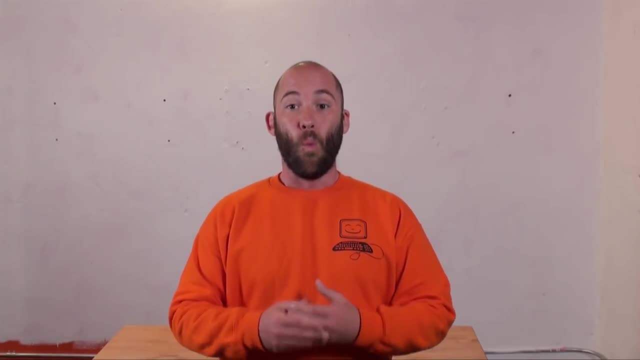 File servers. again, this is just shared files on the network Web server, so you either use something called Apache or IIS to provide websites to people that go to your server, Just like this website here. Almost always, if you have a web server, you also have an FTP server. 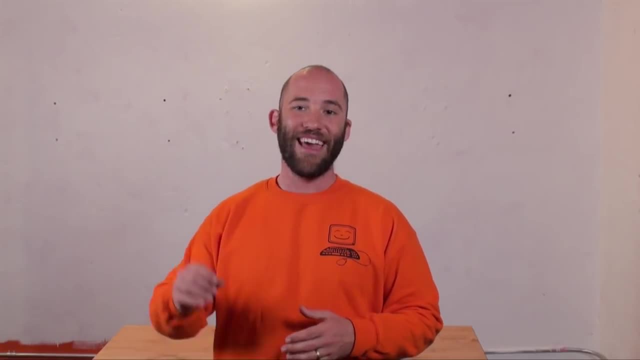 This is a way to transfer files back and forth over the internet. It does so in a different way than a normal file server does, So they kind of do the same thing but in a different way. So an FTP server is different than a file server. 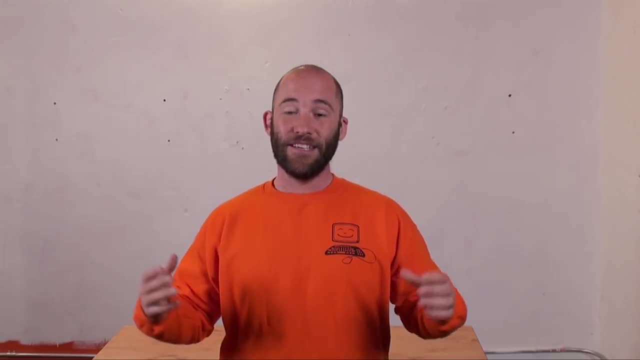 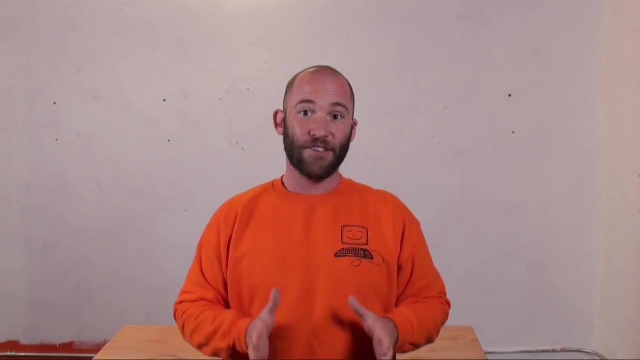 That's very important to remember. We talked about mail servers. These are simply servers that route mail for an organization, So all the email for an organization comes into one server and then that server decides what to do with it. So many times the server will have spam filters built in or it'll have like a Blackberry enterprise. 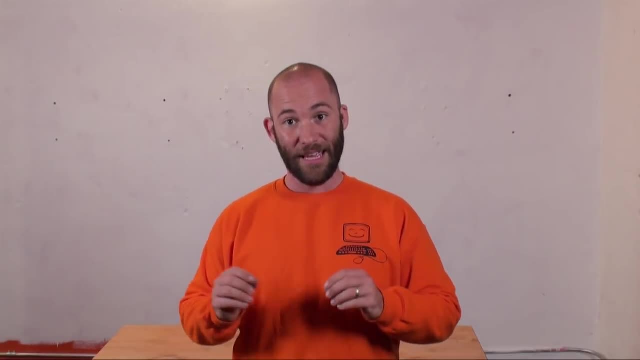 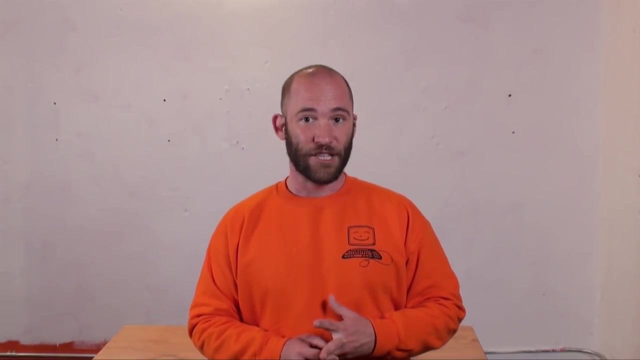 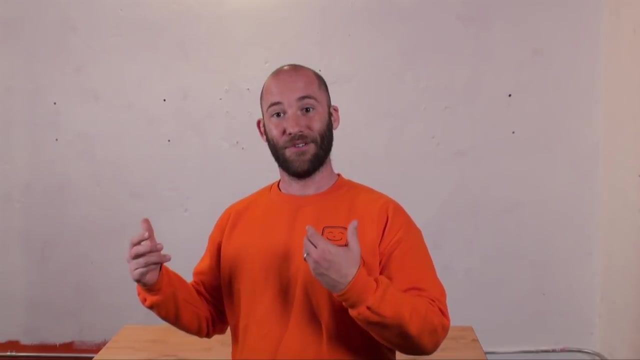 server built in so it'll filter out the spam and then it will send emails to the appropriate Blackberry devices or smartphone devices- Again, the most popular mail server out there is something called Exchange, Microsoft Exchange server. This is a Microsoft product and, of course, can only be installed onto Microsoft servers. Can't be installed on anything else. There are a slew a lot of other mail servers out there on the market. Some can only be used on Windows, Some can only be used on Linux. Some are free, Some are very expensive. So if you don't want to use Exchange, you just got to go out there and use it. 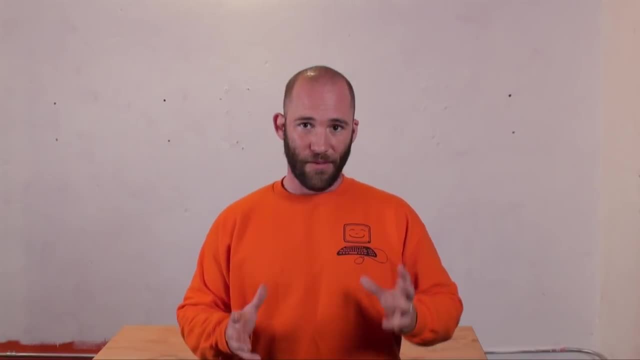 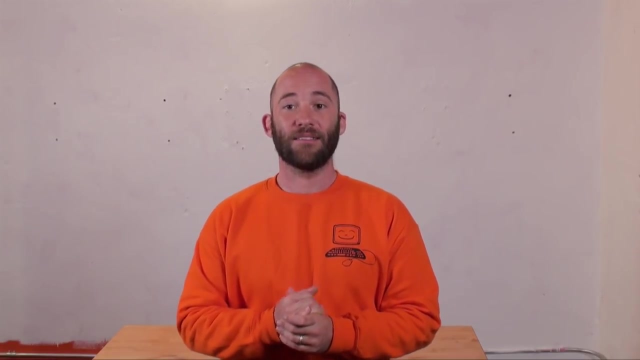 Do some research. Talk about database servers. Database servers: all they do is they just store data, and they store it very, very, very well. This is used for things like contact database systems, ticket management systems, et cetera. And then, finally, we talked about the remote access servers. 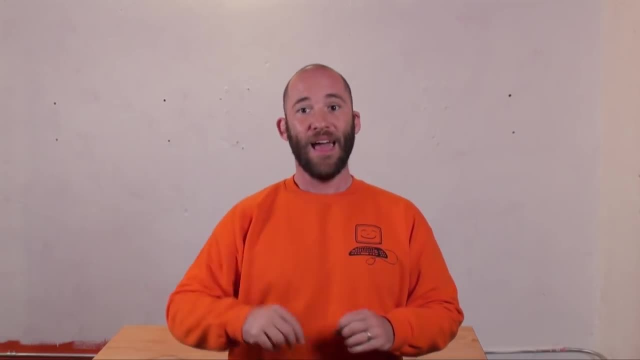 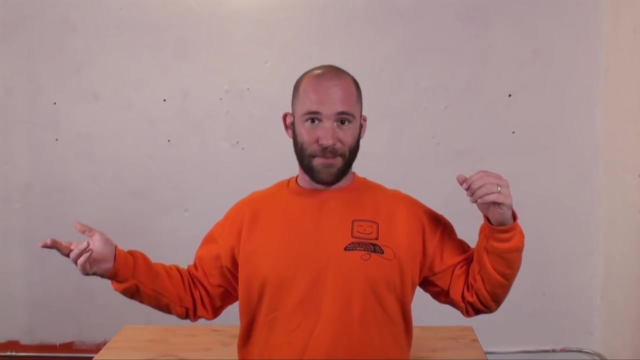 These are the servers that allow people from the outside world to connect to them and then use resources on the internal network. So basically, you know you're sitting in Bangkok, You need to use something that's local And in an office in New York, you use VPN- virtual private network- to connect to that. 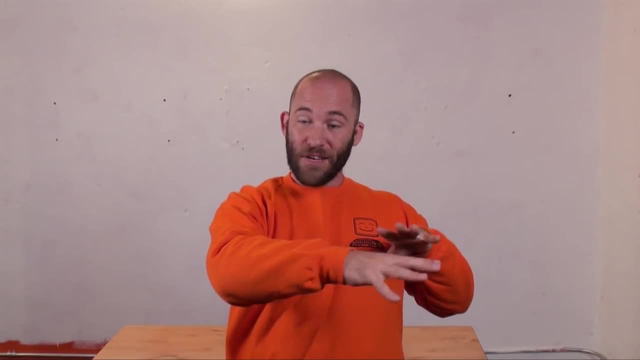 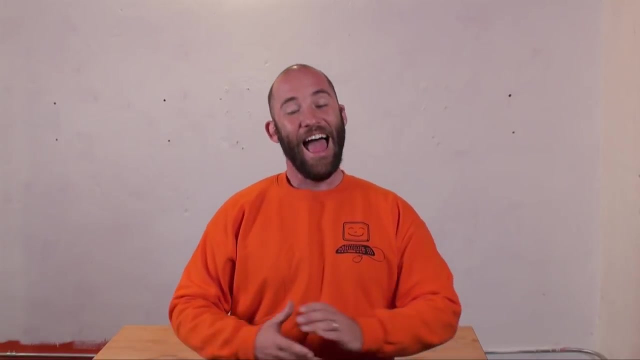 New York office And then you're able to access resources on that local network as if you're sitting there just on a little slower connection, And that's really. that's the introduction to servers. This is going to be a long, this is going to be a long track. 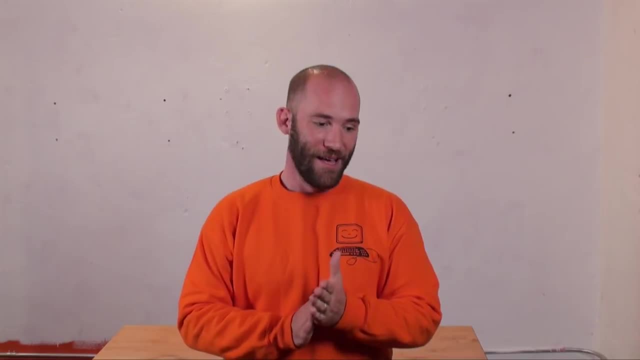 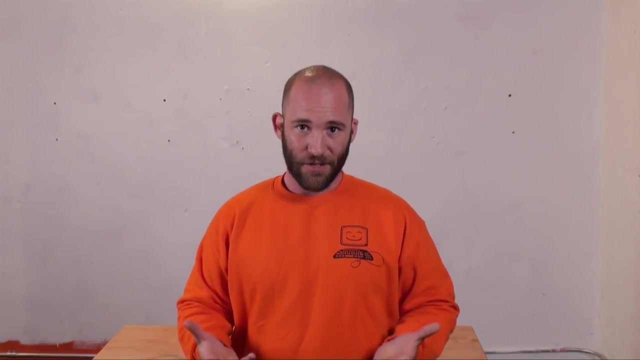 It's going to take me quite a while to fill out, So don't feel bad if this seems a little confusing right at the moment. Okay, So I just wanted to give you this brief introduction, just so you can start getting your head around what servers are. 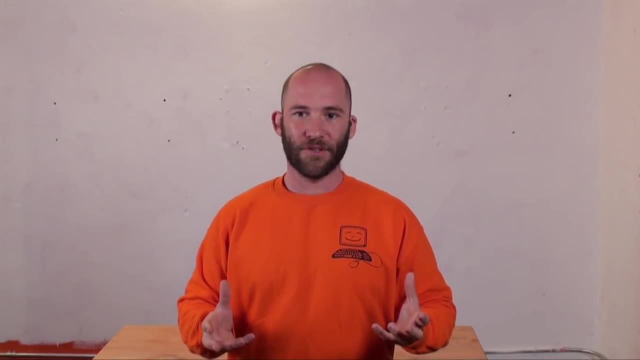 Because, like I say, most people learn about servers from vendor specific classes. Like I said, when I first learned about servers, I only learned about Microsoft servers. I had friends: all they learned about was Novell. I had other people: all they learned about was Linux. 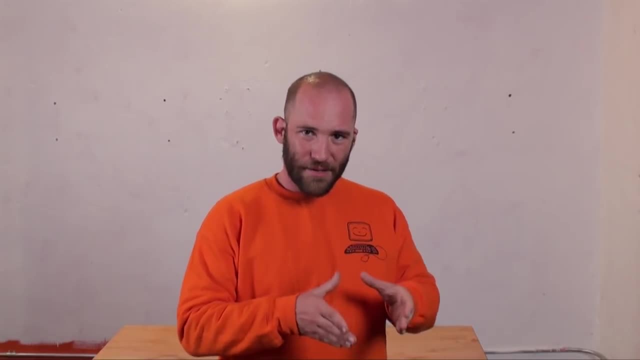 And so when you're so specific on the products, you don't really get such a good idea on the larger world and how everything else works and what options that you or your clients have. The real world advice that I will give to you- that I've seen happen far too often- is: 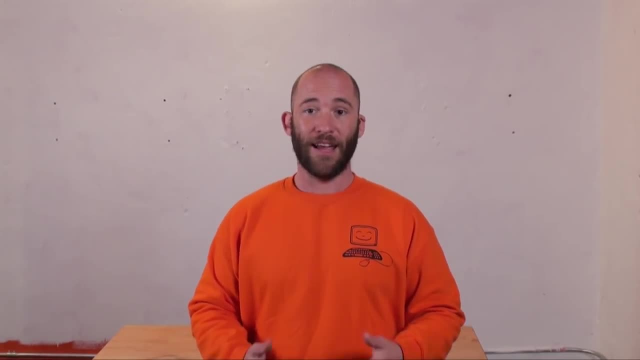 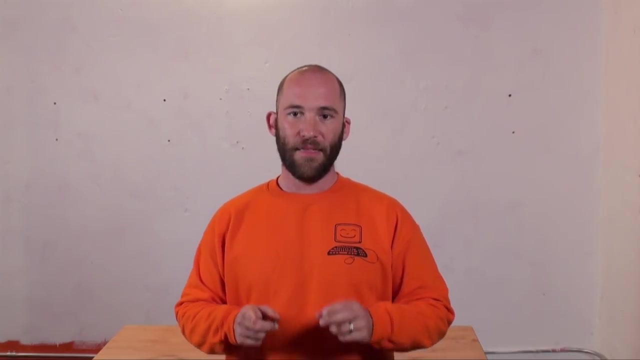 if you have a special piece of software or your client has a special piece of software and you're told that it needs to run on a server, make sure you find out what the people mean by server. I have seen a lot of servers that run on a server. 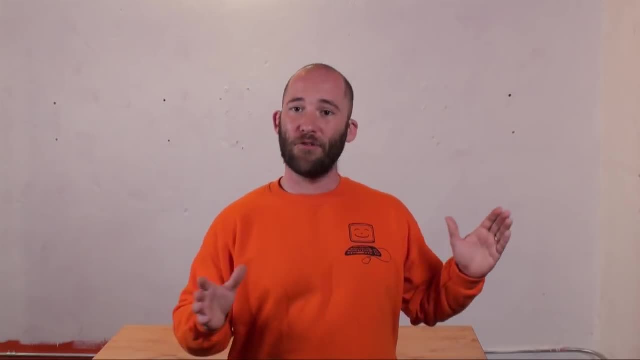 I've seen a lot of people when I had the repair shop that they would go out and they would buy these $4,000 and $5,000 servers because they were told they needed a server in order to run some piece of software. These servers were very expensive. They're more expensive to maintain because you do need to be certified, You need more knowledge to maintain them than you do to maintain a desktop computer, etc. And then when I would call whoever created the program and just trying to figure out.